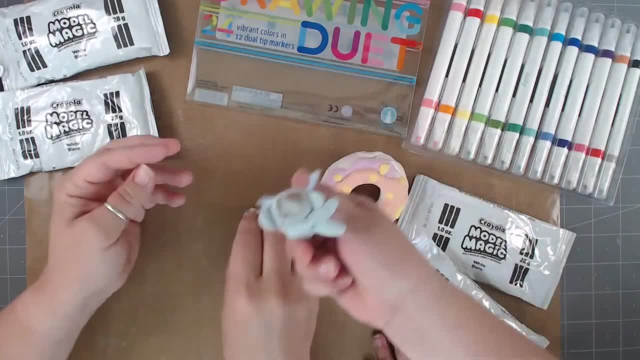 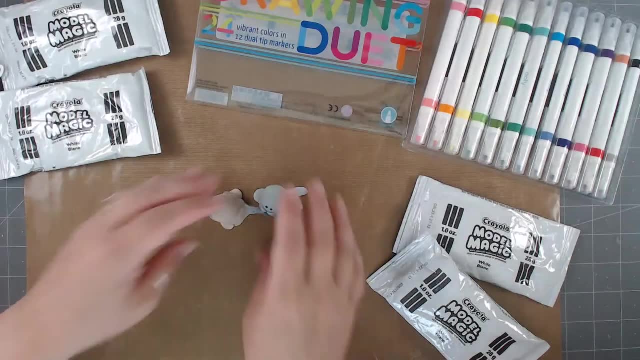 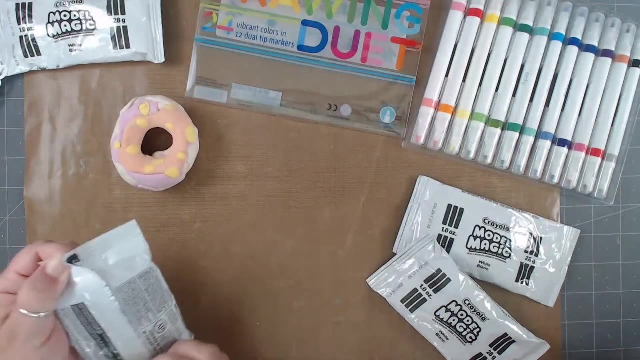 tail got torn off, but you let these kind of sit and they're very, very lightweight. I mean, they're super, not heavy. Even a baby can pull these. And is this clay fun to play with? Yes, All right, so let's pull the clay out. You open a package and I open a package. Do you need scissors? Okay, 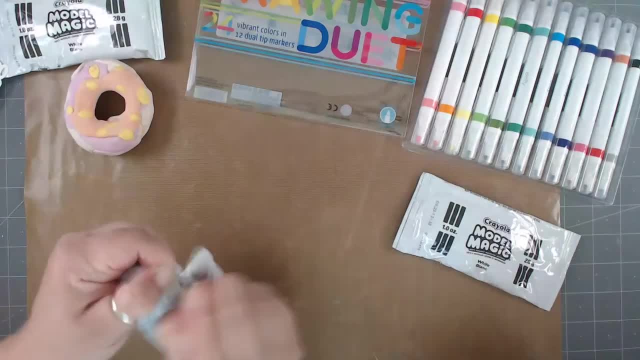 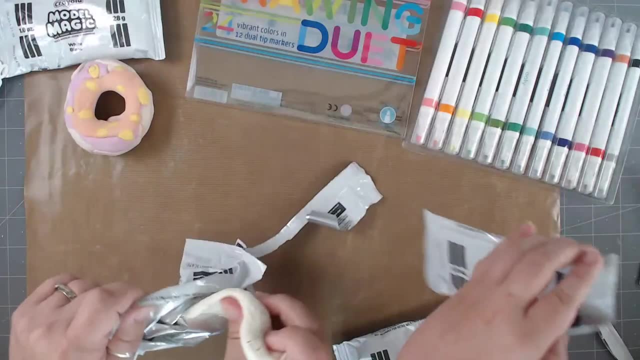 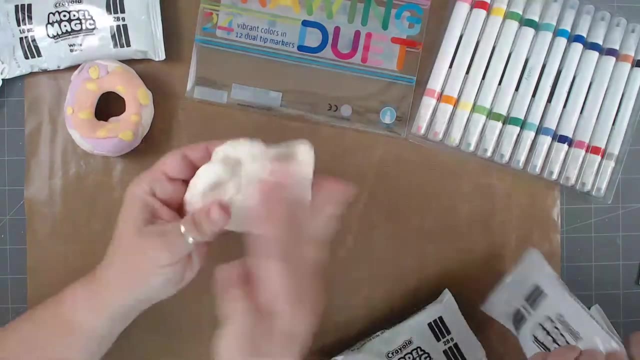 So they come in little one pack, one ounce packages, and it comes white. Now, this stuff is so fluffy and so cool, So it comes white. so you can like change the colors. You can change the colors, Exactly right. So it's just. it's stuff is so fun to play with. It's just, it's like playing with. 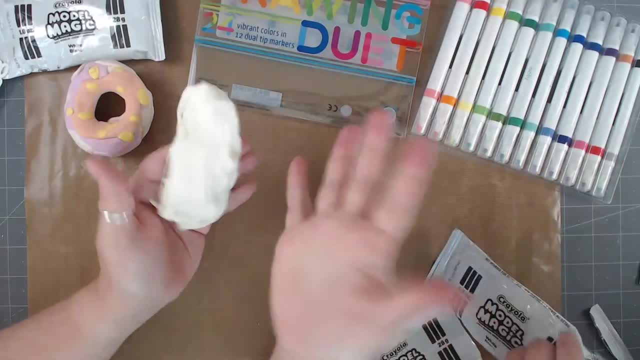 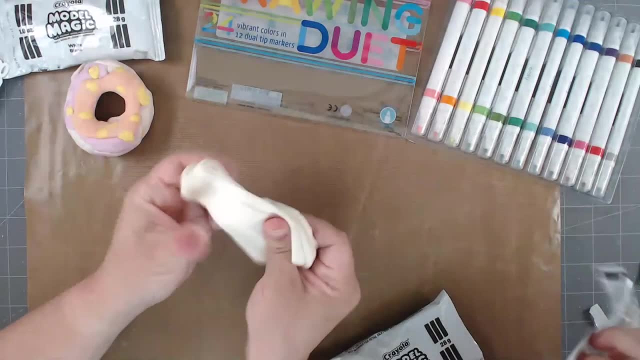 marshmallows Or playing with slime, But it doesn't stick to your hands, which I think is awesome. Yeah, it's kind of like a fun slime, It's like the fluffy slime, But if you leave it out to the air it will dry, which I think is awesome. If you put it in a container so that it seals, it won't dry. 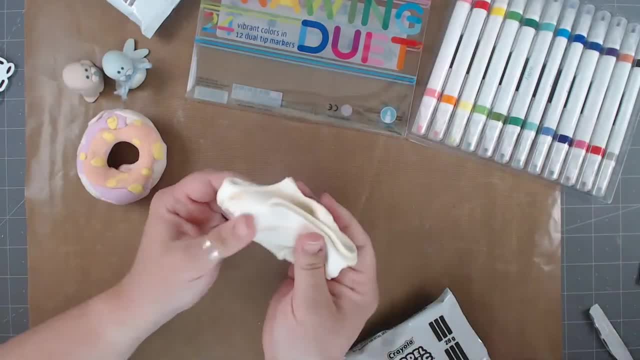 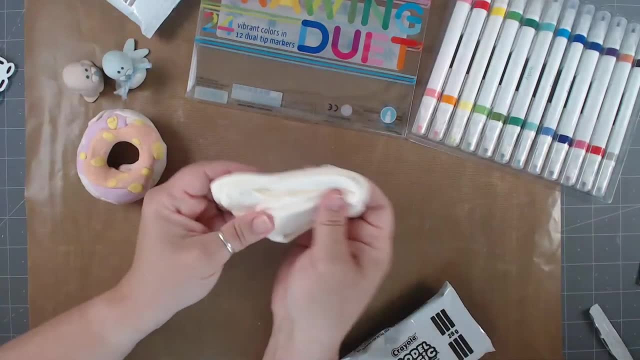 Right, So if you put this back inside like a Ziploc container, as long as you don't get it too mucky, gross, then you can reuse it over and over. So I like just playing with it like this. Pretty fun, Don't you? I'm gonna split one of these so I can make different colors. All right, So I'm gonna. 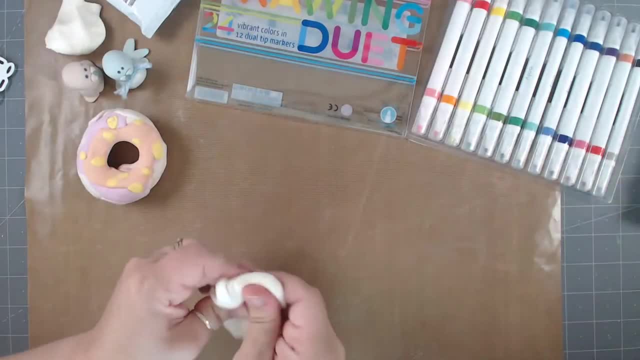 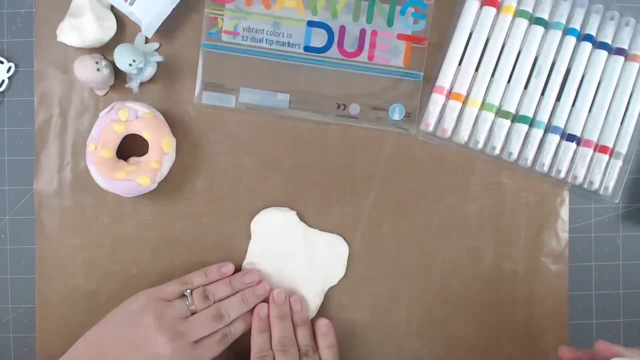 show you, guys, how to color and color Heather, what color are you gonna do? I'm gonna make my donut first, So she's gonna show you how she made her donut. and I'm gonna show you how to make a little animal, So I'm gonna pick the darker pink color and really, truly, you can go any color you want You. 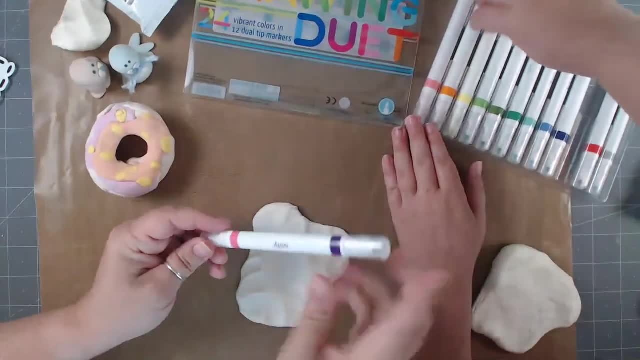 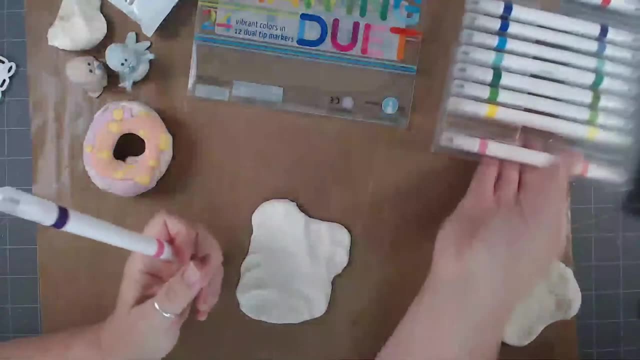 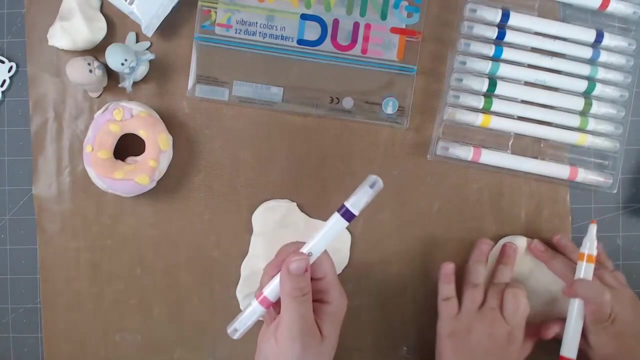 can also blend colors. So if you look at these, there's two different colors on each end. So you actually get a lot of colors on here. So I've got, if you want to see we've got. okay, so what colors on the other side of orange, Red, We got red and orange. So you're getting 12 markers but 24 colors. 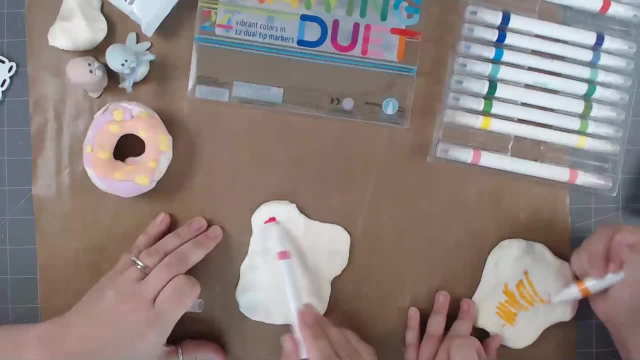 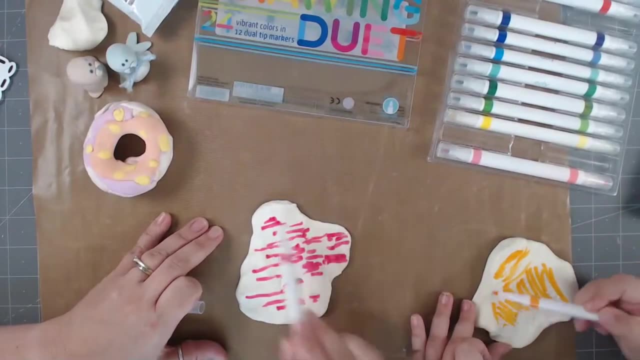 pretty darn awesome. So we're gonna do pink and, just as she's showing you, you're just gonna come in And draw And you just color on it. You can draw, you can color or you could draw like some figurines. I mean, you can have fun with it. You can also make your figure and then color over top of it. So we 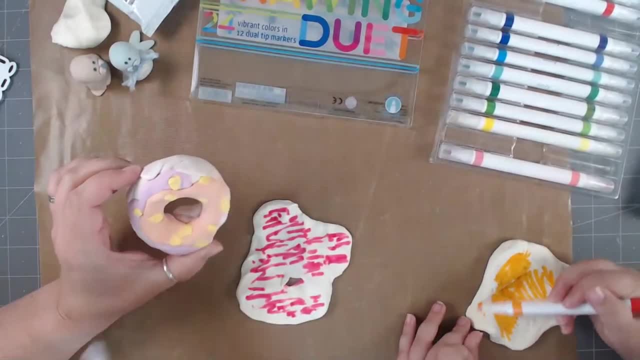 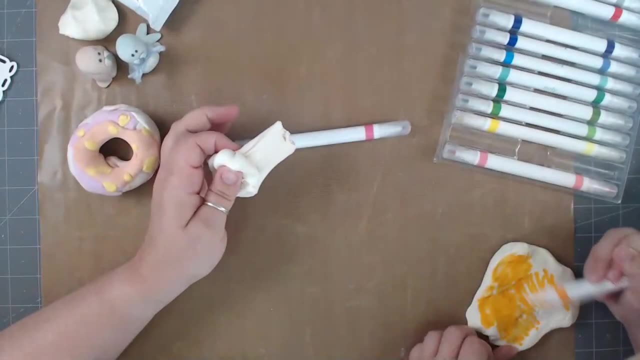 could go in now and we could color over top to add more sprinkle colors. right Yeah, But I'm not doing that because I don't think it looks good, Totally fine. So I cap my marker and I'm gonna move this stuff to the side. So we got some more room. 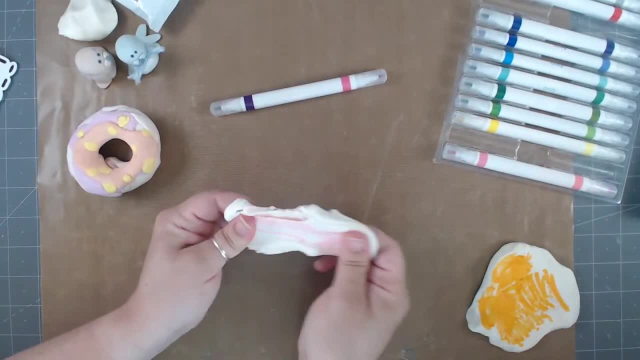 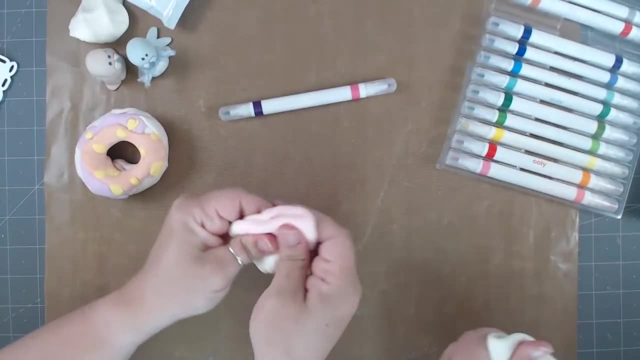 here. So I'm gonna cap my marker. You can also use paint, Exactly right. So you could do this exact same thing. add a couple drops of paint and just go from there. So here I am, I'm blending it in. Look at that, So you're gonna get a very Lighter color than it. That's exactly what I was gonna say. Your color is not gonna be as vibrant, It's gonna be a little bit lighter. 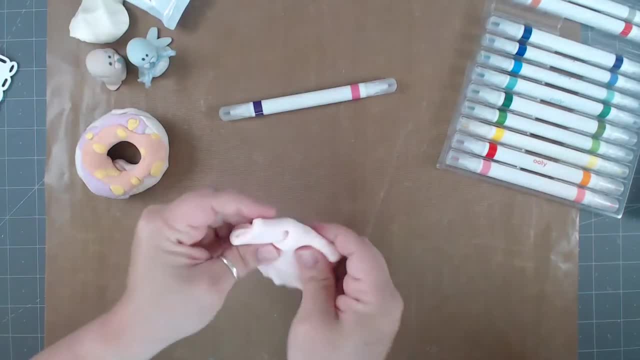 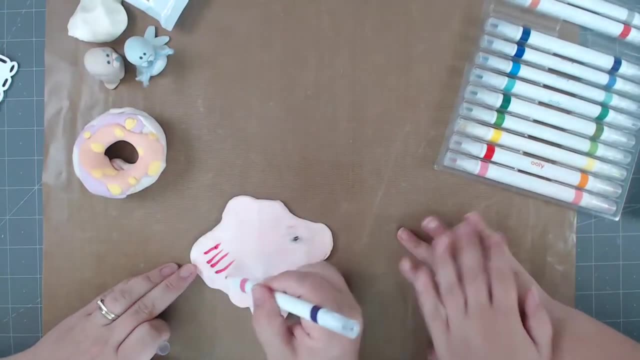 And you add more color to it. Exactly So like this is just a little too pale. So I'm gonna flatten this back out again And I can't even see the orange. I can. but it turns out like this: It's a little bit darker. It's a little bit darker because it plays white already. 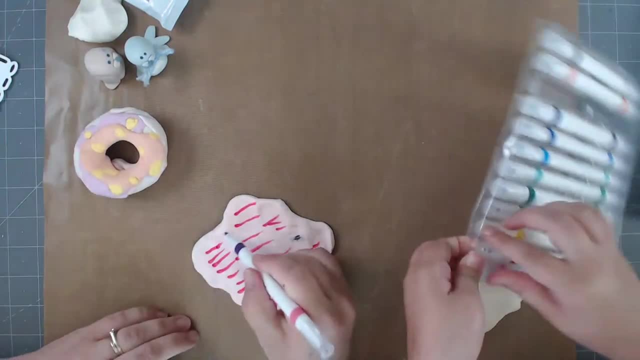 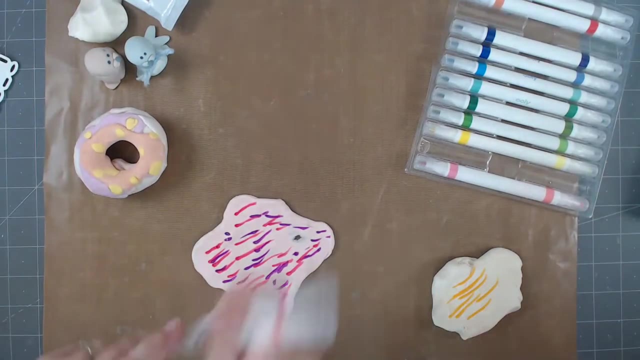 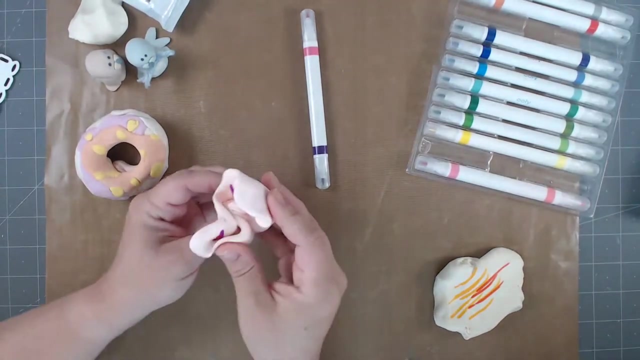 There we go, So I'm gonna add this and then I'm gonna come in and actually add A little bit of some purple Just to give it, So you can do more than one color and you can kind of play around. It's because orange has got red in it, right? Yeah, That's how you get orange from red, Yellow, yellow and red. Very good. 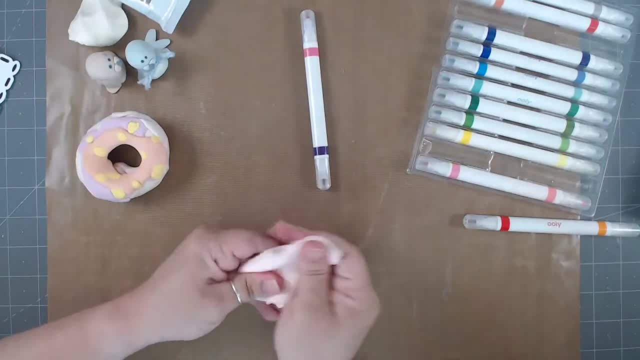 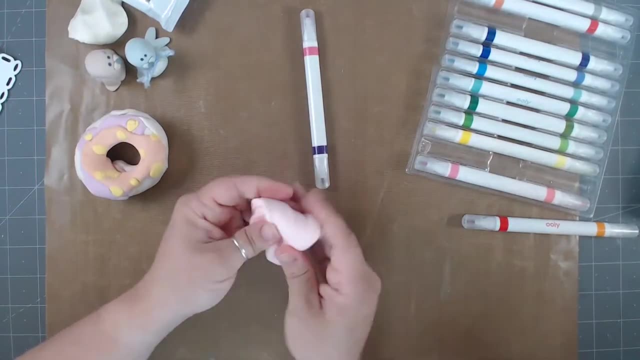 So this is a great way for the kids to do a couple of different things. This is a great home activity One. they're getting very tactile and they're learning how to mix colors, mix colors to create their own colors, and they're also learning how to work with sculptures. they're working with 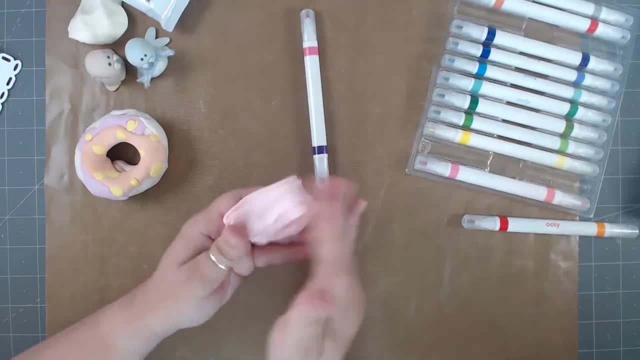 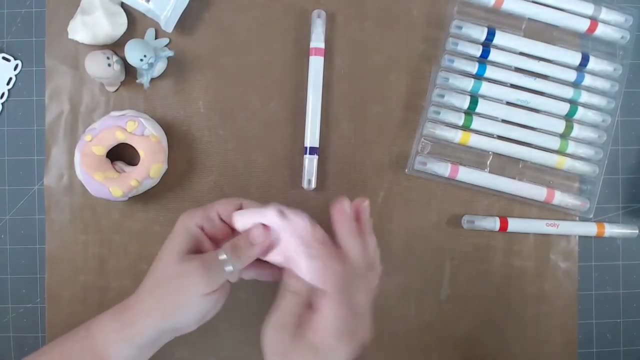 making, creating objects. so the little bear I'm gonna show you guys how to make today is actually a really, really simple, because it's just a bunch of circles and just putting the circles together. the doughnuts are really fun too, but think about all the other fun things that you could make. I mean you can go with. 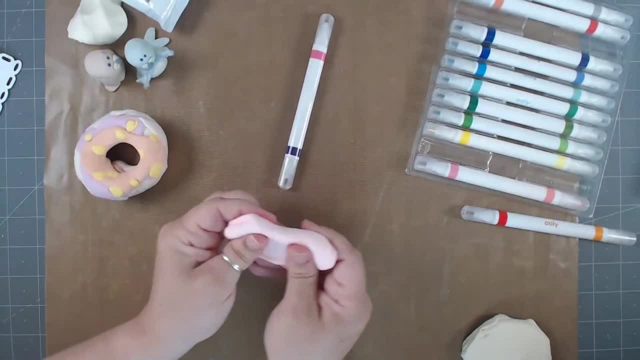 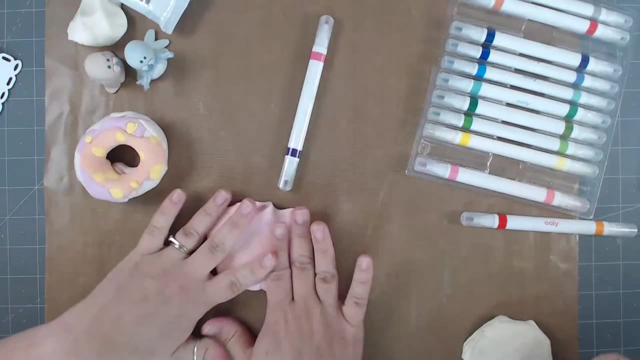 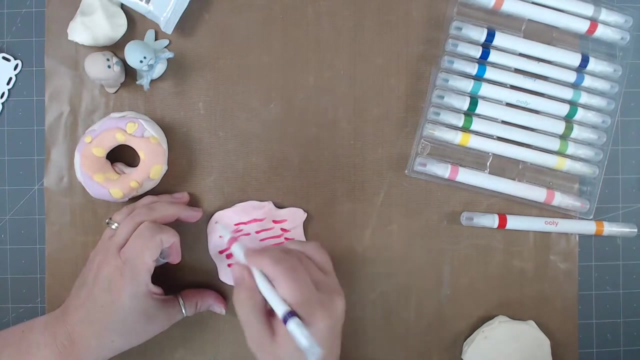 animals. you can make flowers. flowers are really pretty. so much fun. just keep blending your colors. I'm gonna go a little more pink. why are you opening up? another? one doesn't need the frosting and the sprinkles. okay, that's why I need to. this is, hands down, one of her more favorite things that she's gotten out. 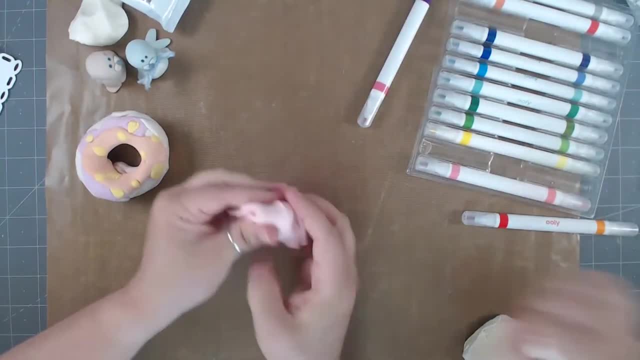 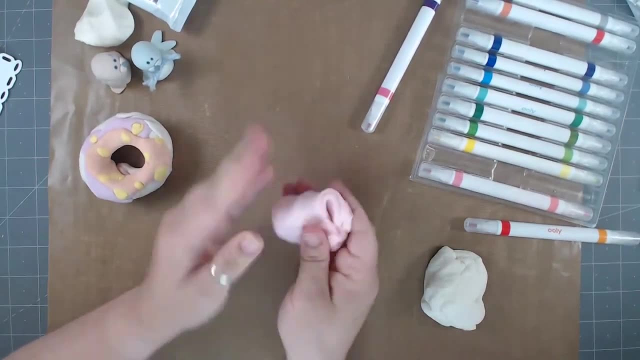 of the orange art box is this clay. she thinks this stuff is awesome and I believe they've put it into a couple of different boxes because I'll suck you with it for a while. I get softer and fluffier it. yeah, it does, because you're. 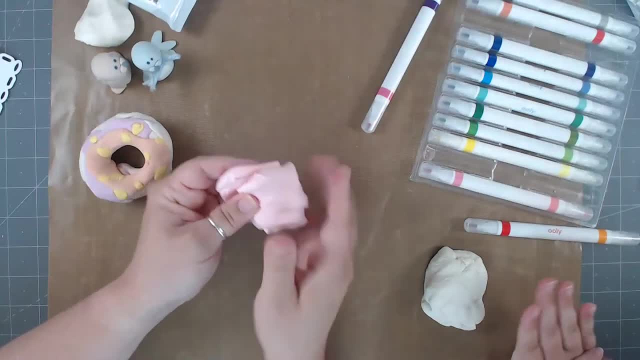 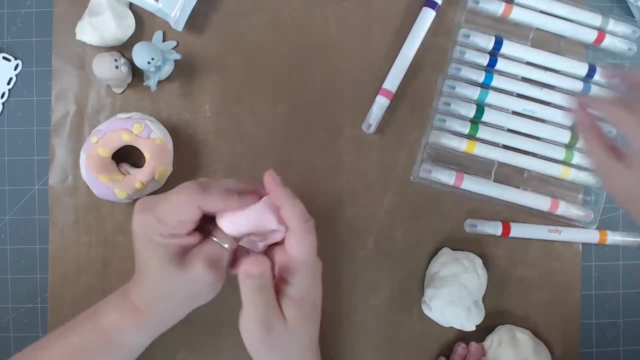 kind of warming it up a little bit with your hands. but I know that that orange, our box has put this clay in a couple of different kits because it's just been so popular. it's one of the hands-down best things that they've put in their box. I 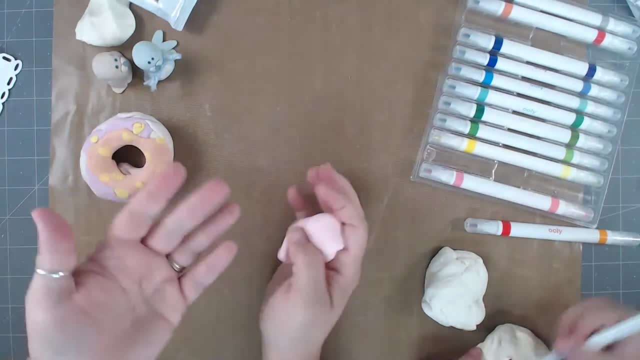 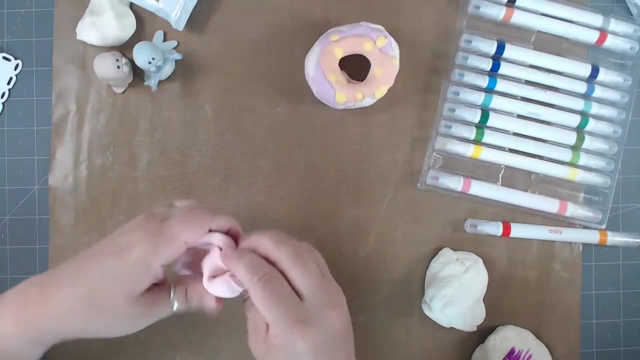 think, because you can go any direction with it. you can stick with the theme of the box. for instance, this one's in the dinosaur box right now, but you don't have to make dinosaurs. you can do whatever you want with it. okay, so to make our little bear. what I'm gonna do is I'm going to 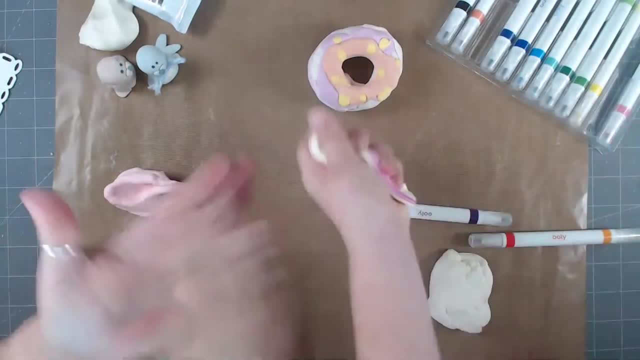 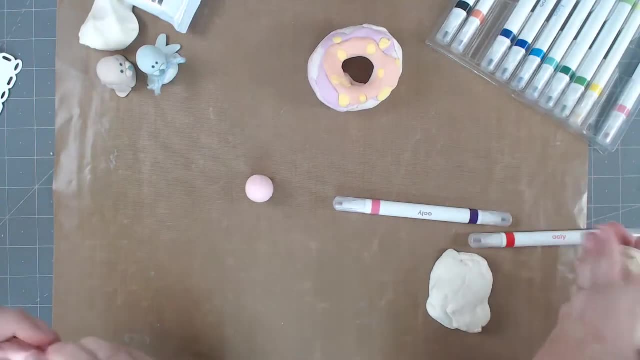 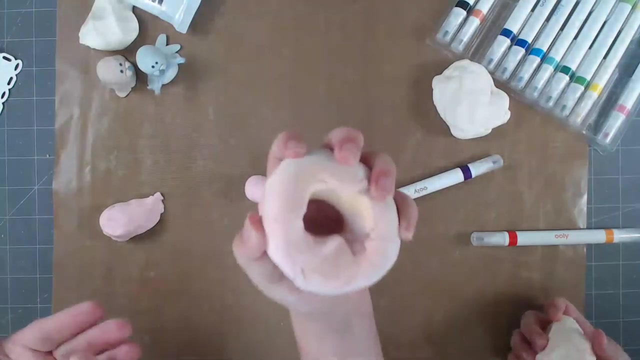 come back on screen- a little bit off screen, because I'm gonna roll this and I'm gonna roll and make little balls, right. so that's my first one, and then I'm gonna create another one. so I'm gonna create another one and I'm gonna show you how to make the doughnut hole, like how you make the base of it. oh there. 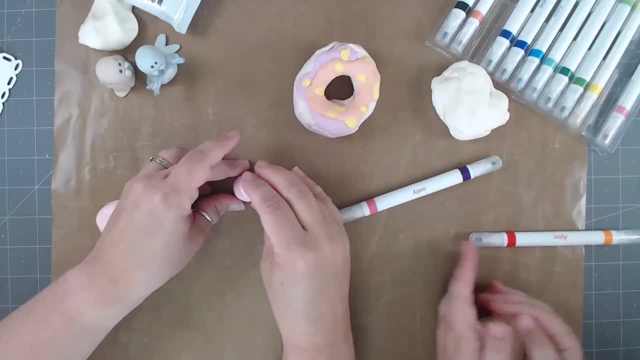 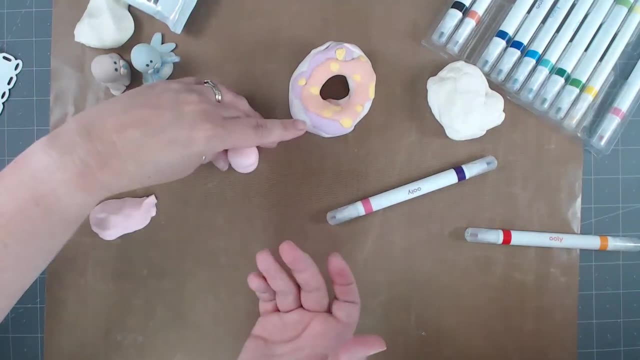 you go. so I've got a couple of different balls, and then you can place one ball on top of another. there we go, and that's the beginning of creating your little guy. so so far super simple. it's just making it smaller and bigger, and then we also make the ears right. so now I'm going to 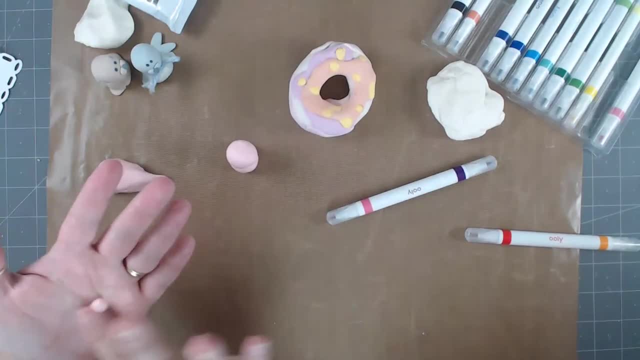 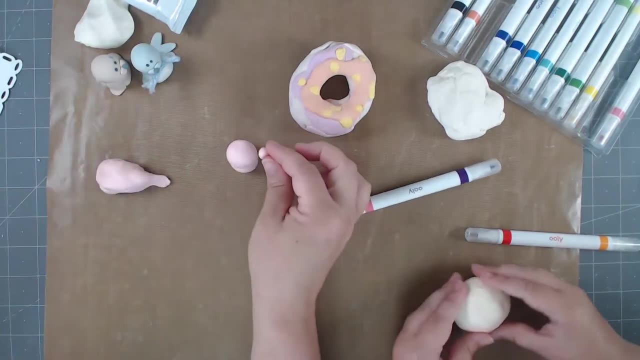 create a little ears. so I'm gonna come in, go, okay, is this gonna be about the right size for an ear? so I'm just rolling it mine. hi e-squared, hi Sue. okay, there's, that's what I do, kind of like push a hole in the middle and it. 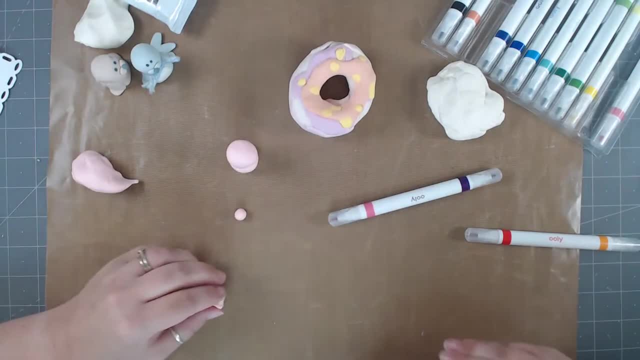 kind of makes like a doing that shape. do you wanna make that more colored? no, no, that's kind of cool. so she didn't fully blend in there. okay, I didn't fully blend, marbly, look on it, Very awesome. So I'm gonna take another piece of clay and I'm 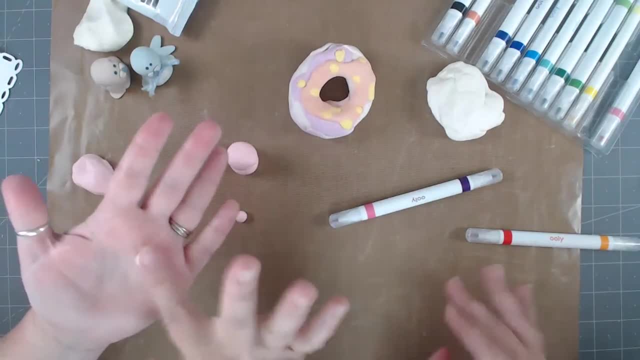 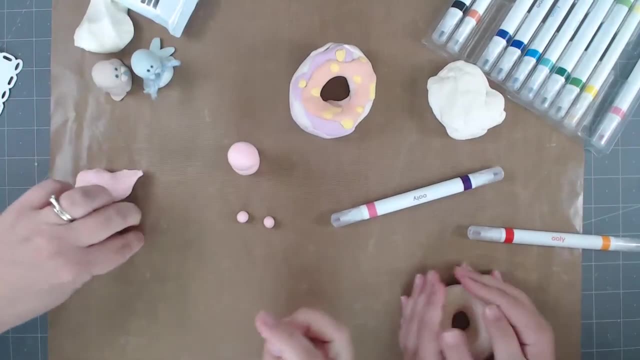 gonna roll it around. So this is just making circles. Could you do little circles like this? So it's just a matter of little circles, And then I'm gonna create little feet. This becomes the ears. Pop my little ears on here. I got the. 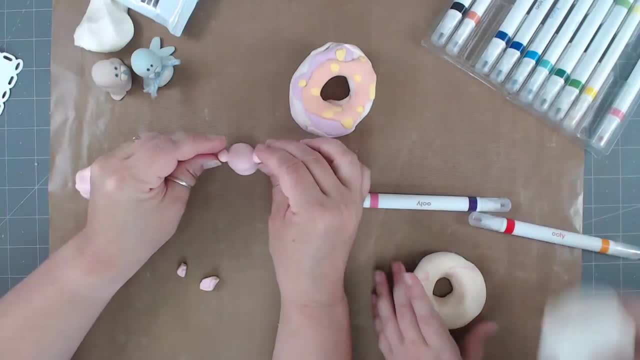 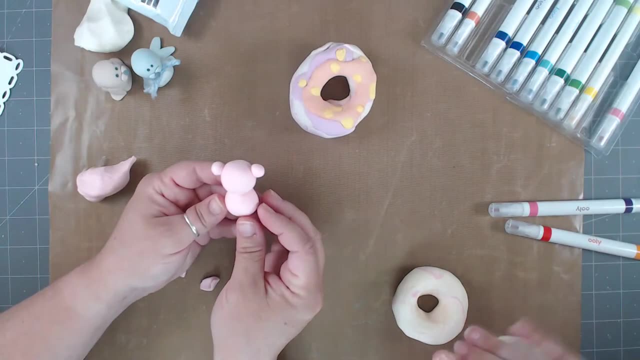 donut shape done. Now I have to work on the plastic. I want your donut to be a little big, Right, So you can already start seeing a little bit of a bear showing up, right? Yeah, Looking kind of bearish. Yeah, Don't forget about the. 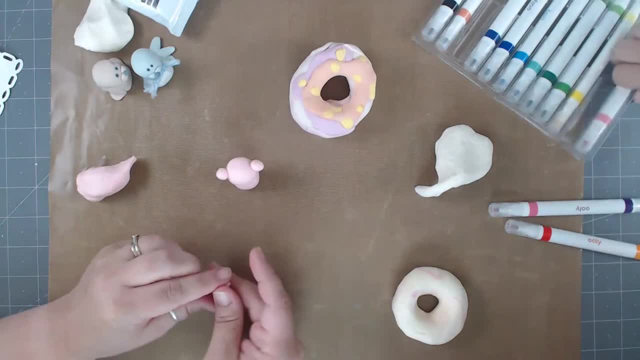 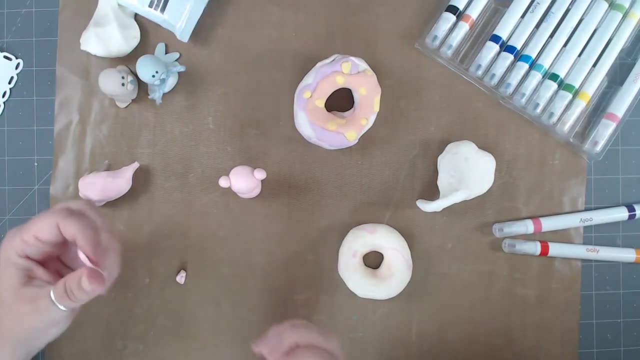 muzzle, I'm getting there. I'm getting there, That's coming. Yeah, her little donut is pretty darn cute. I have to admit I love the marbly. look, That's pretty cool. Alright, so now I'm gonna make the little feet So you can either roll it in your 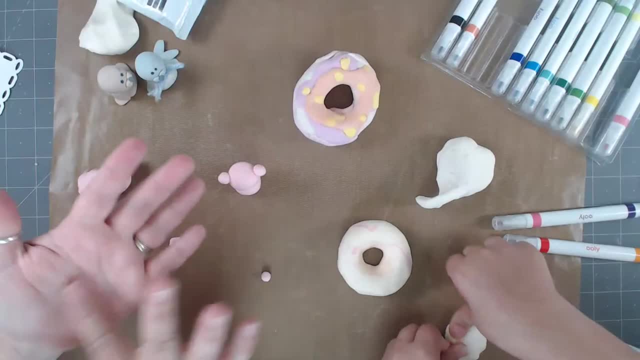 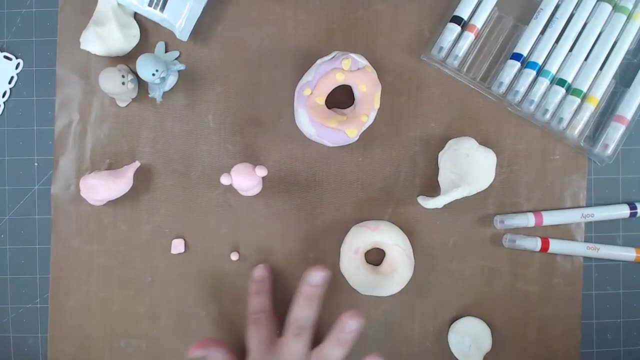 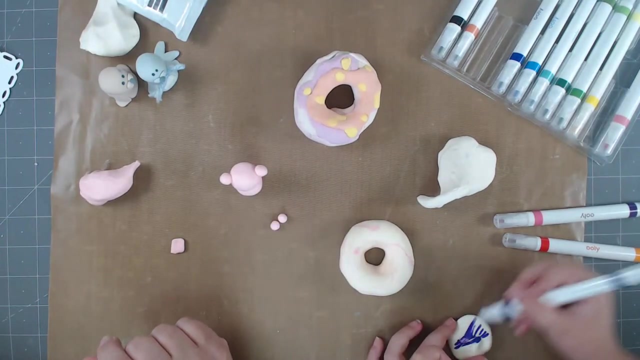 hand to make little pieces, or you can make large stuff. So I mean Also, if you have like some like type of like color on your like desk or something, the clay will pick it up. And what else will the clay pick up? Burr dust, dirt, So we put. 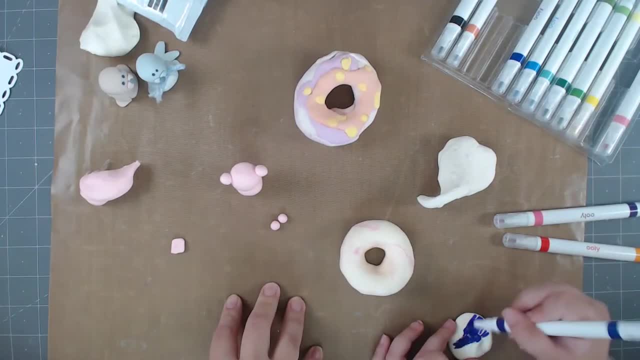 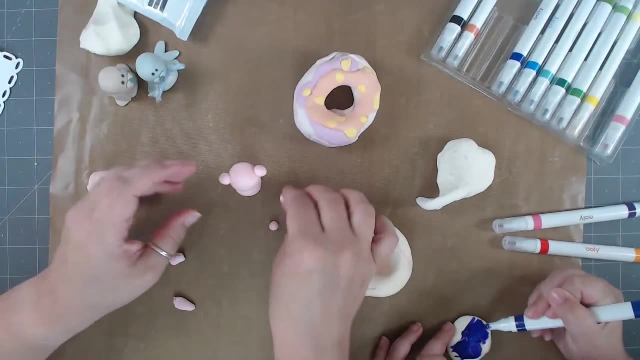 down a clean craft mat that we just kind of. I just washed this the other day, So that way it doesn't have those problems. Alright, so now I'm gonna make the little feet Also, so we don't get marker on my mom's desk. Marker on my desk is awesome, So I'm just gonna put two. 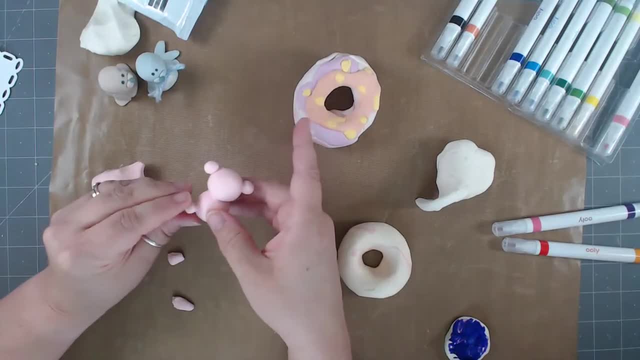 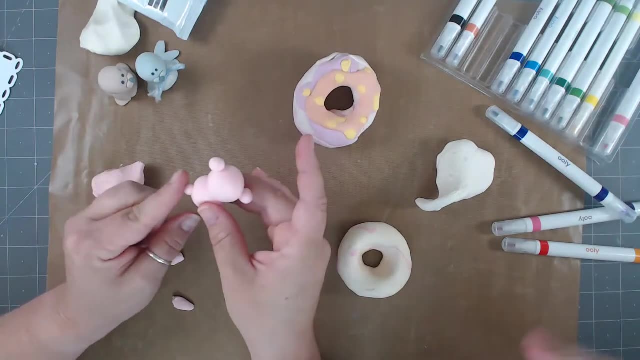 little feet down right here. Pretty sure that's gonna be enough marker on mine for now because it's really small. This is going to be the sprinkle color Purple. So I just Look at the color. it's turning out like It's like turning out purple. 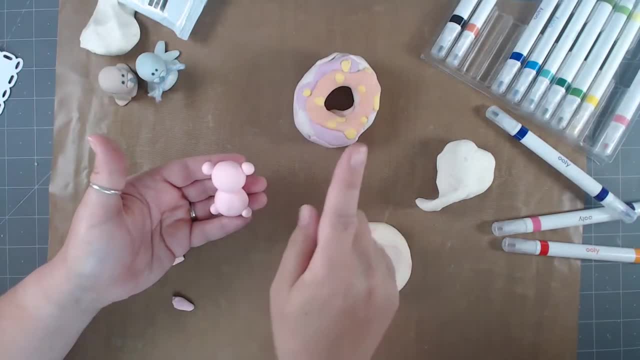 So so far, all I've got, I've got large circle, large circle, That's right. Show them, Look how cool that is, It's pretty, pretty. Water-based markers work on clay- Yep, absolutely, That's what we did I used just to show you, I did not use, I use Crayola. I did not use these markers for these. 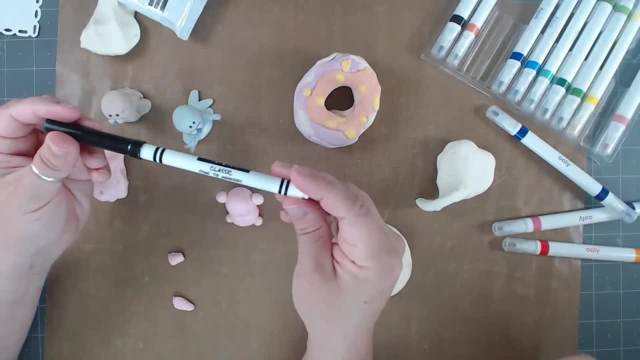 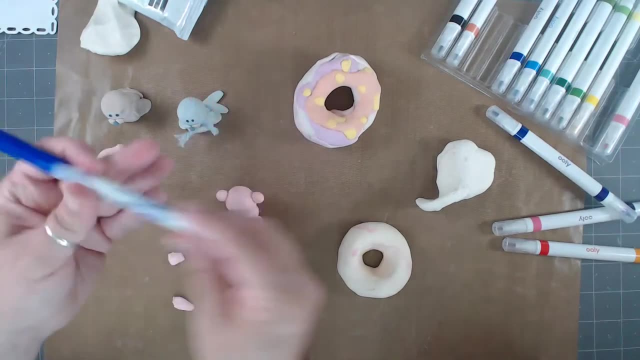 little guys. I use this Sergeant Classic Fine tip black markers And they worked absolutely fine. And for this little blue guy I actually used this dark blue marker. and these are all I mean. so very kid friendly, You could use the Crayola. 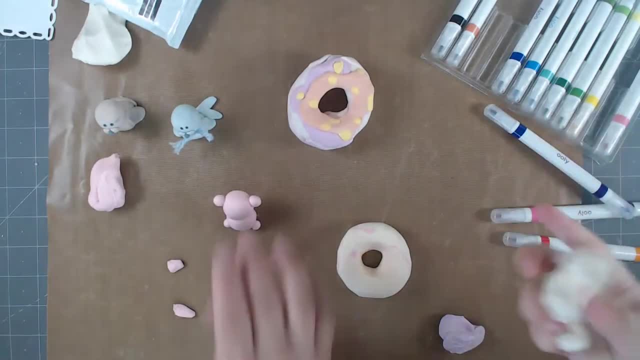 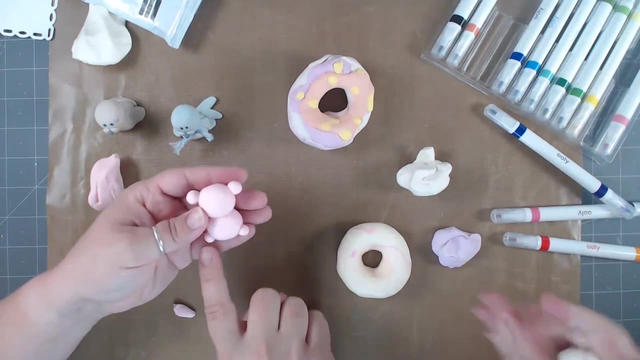 markers. whatever you have on hand. You don't have to use fancy markers and it works great. Alright. so for my little bear, as you can see, we've got the head, which is just a ball, two little balls for ears. 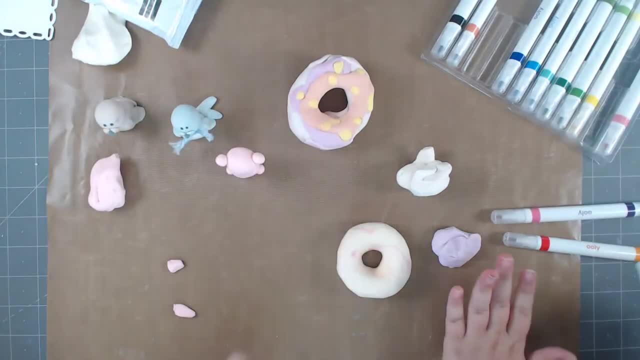 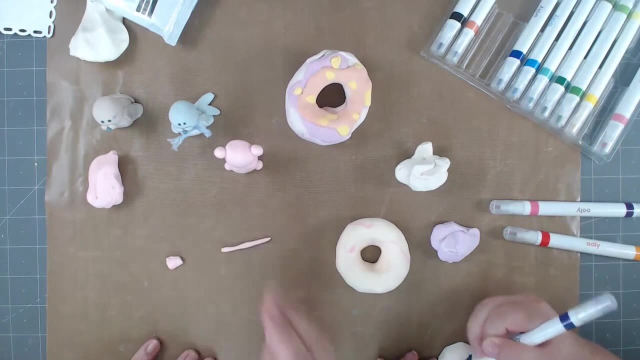 I've got two little feet and now we're going to make the front paw, So it's going to like sitting up. The front paws are little bit different. you kind of create a rope. so so far the shapes we're using are just circle. 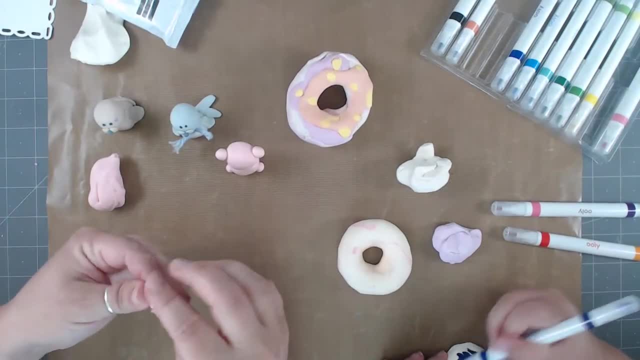 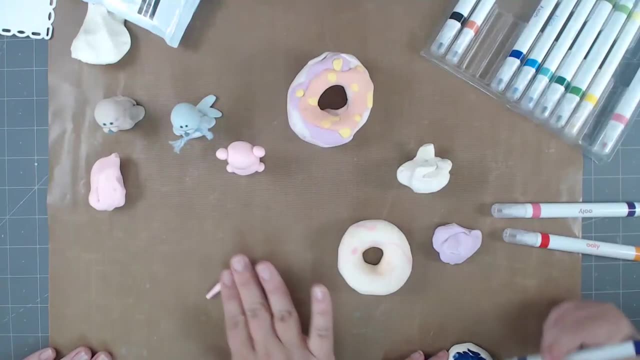 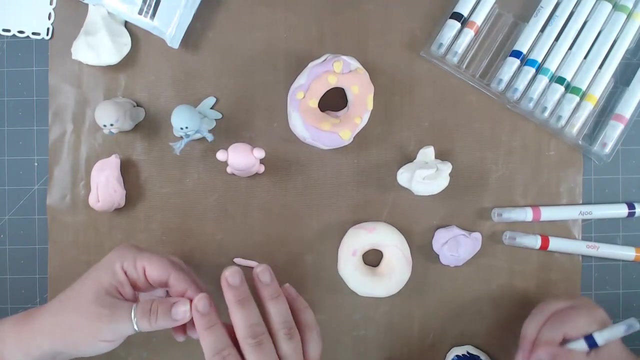 circle rope. not too hard, I'm going to make this a little bit thicker. no, circle, circle snake. if you want to, okay, yeah, okay, if you want to call it a snake, you can call it a snake, or worm, or worm, sure. and sometimes I'm like, oh, that shape was not the right size or that was not quite the right. 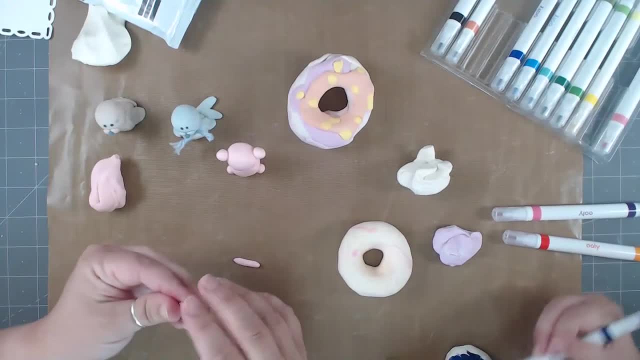 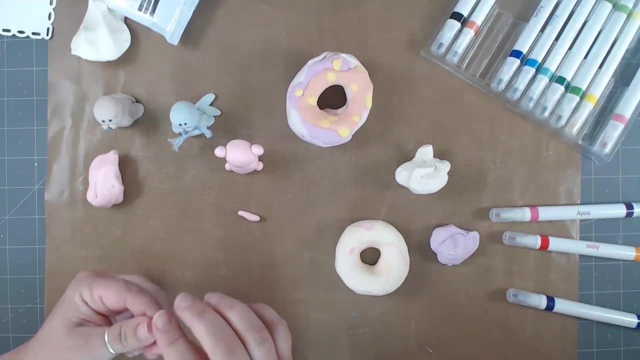 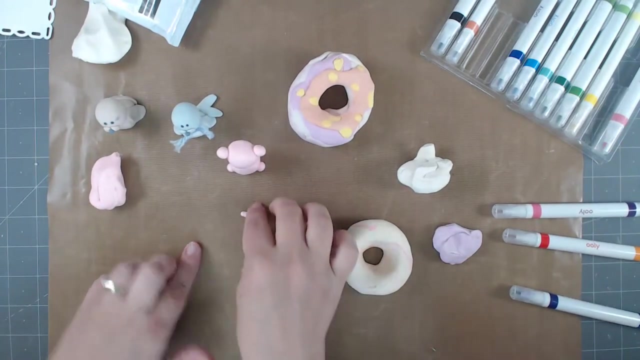 scenario. so I'll readdress that. so I'm just making the little paws the front paws. yeah, I'm just calling my thing blue because I want like a dark color in my frosting. and what if you mess up? do you have to like you can just tear it off and start over the best part, because it has it's not? 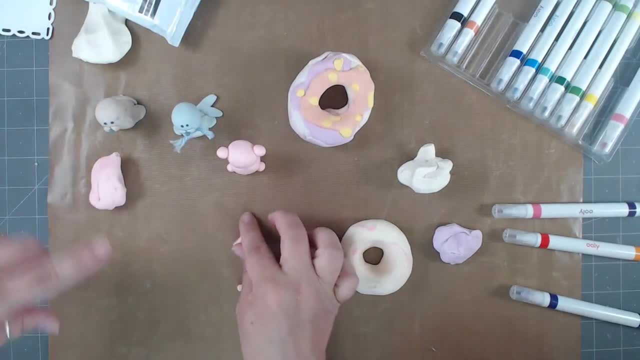 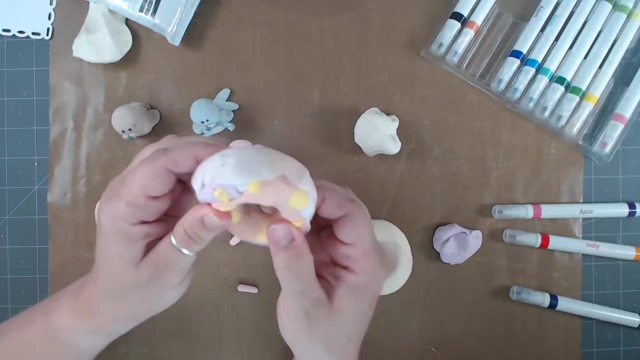 like it's. once you've set it, it's got some time, so air drying from making this little guy to when it dries over here would probably be a few days. well, overnight, I would take it overnight if you really want it to be hard, like these ones I made back in December. Catherine, you made this about a week ago. it's still. yeah, it still. 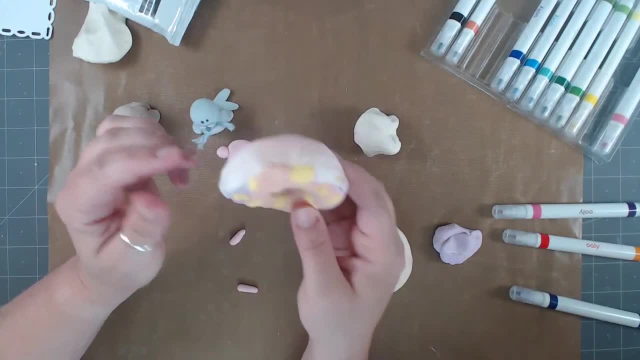 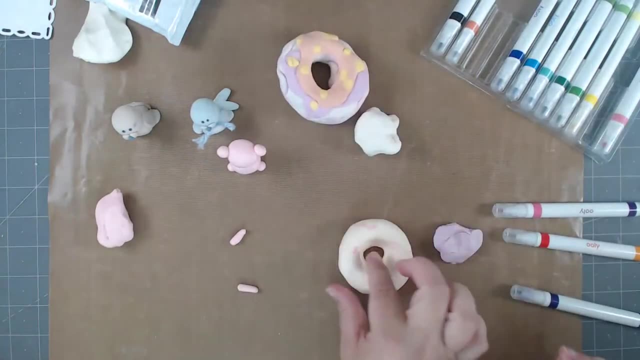 has a little bit of some squish to it, because if this is really thick, so the more clay that's in there, the longer it's going to take to set. but you can't take this back and go to here. it's like it's not going to happen. all right, so now we're going to get our little. so, if you notice, I've got two. 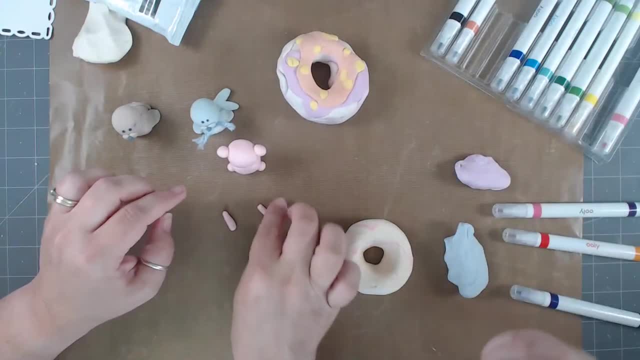 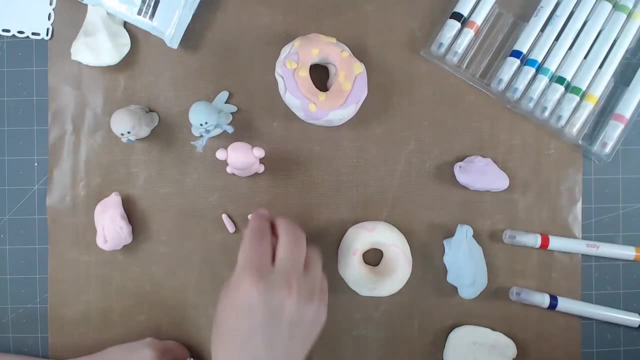 little arms. I have purple and blue. I have purple and blue and I'm making the other half of the frosting cool, which is going to be like a different color. I like your color choices. they're really pretty. so I made two little arms and what I'm going to do is I'm just going to attach two arms from the front, kind of coming down, cool. 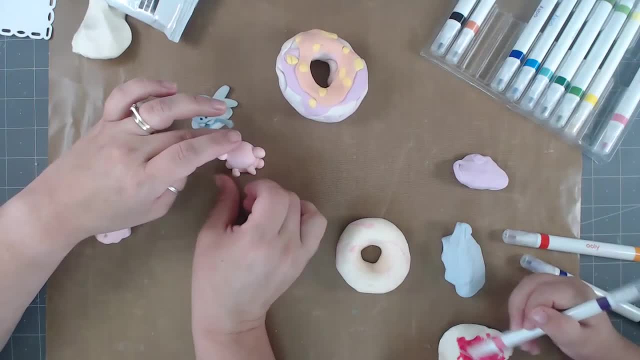 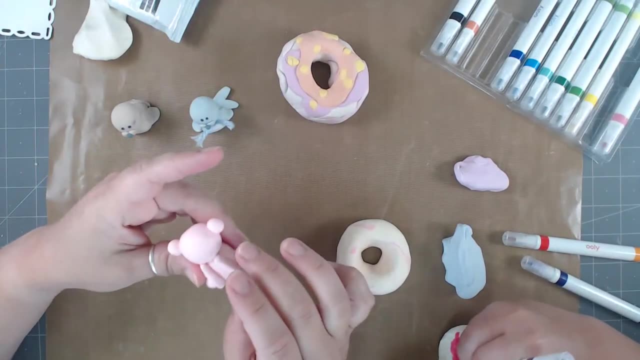 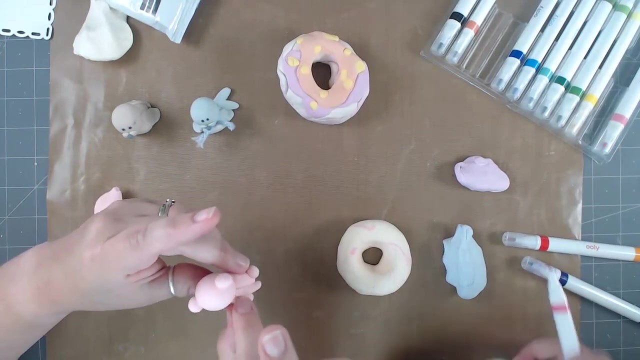 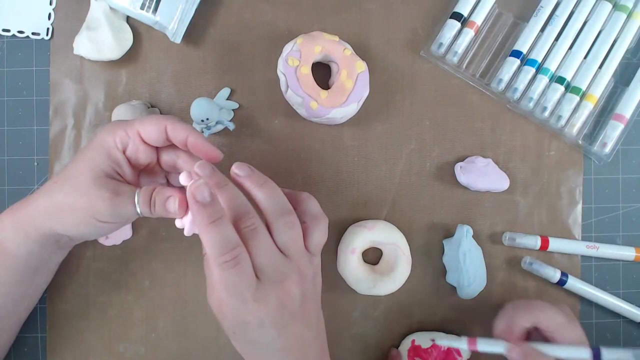 cool, that's cool. also, the marker won't go on soft like really like wet pieces of the clay, like see, look, it's not going on that piece right there because it's wet. huh, it's not going on that piece because it's what do you mean? it's wet. 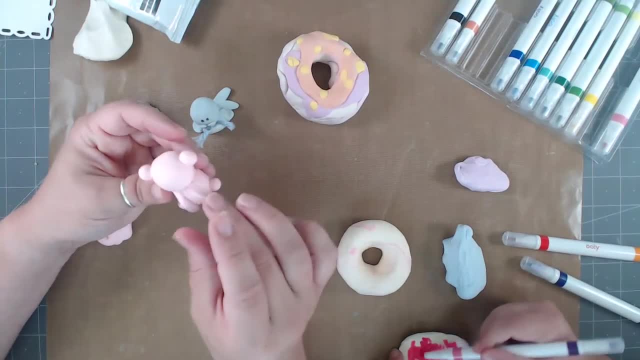 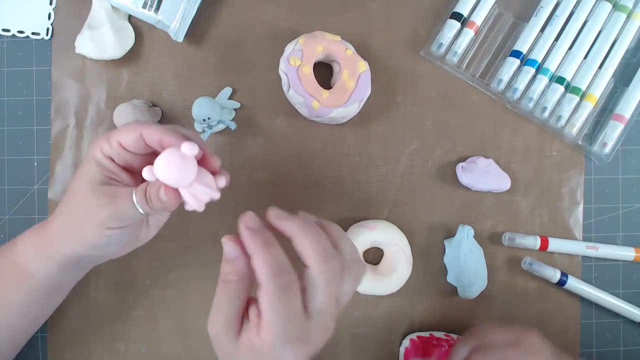 like it's like a little soft. oh, it was overly wet, yeah, got it. that means you can't go on. the water won't go on. so one thing about this clay- because it's so soft- is that you, if you push too hard, you start denting. so I've got a little dents in the back where my 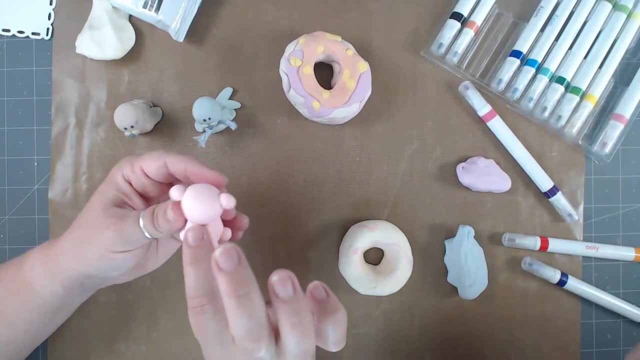 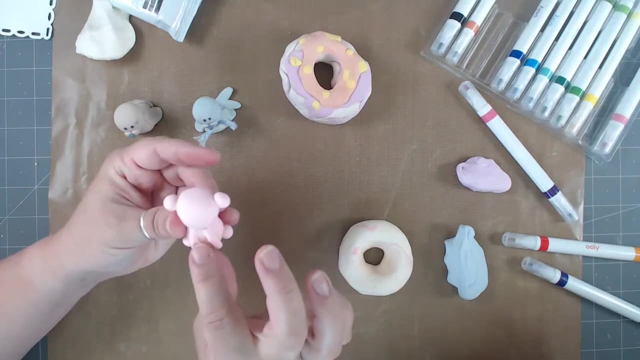 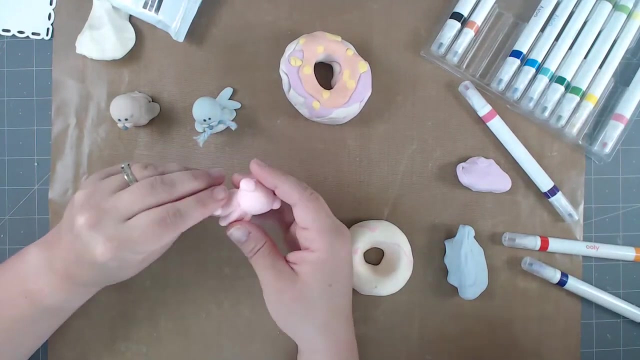 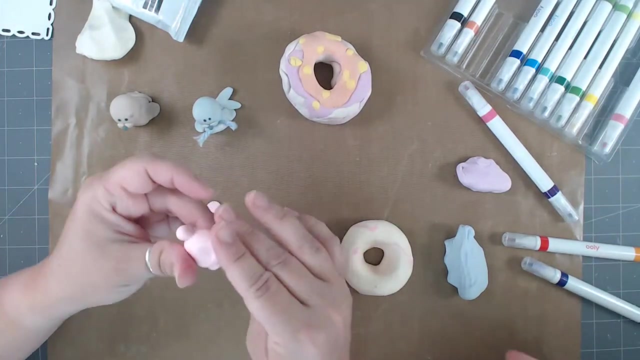 my fingers are pushing on it okay. so, wow, rolling bear. not my best there, but you get the idea. this is the front. so here's his front, little paws and his little feet. you're trying your best, I am, and sometimes I'm like you know what: I'm not a big fan of the bottom. so we're gonna rip it apart and I'm gonna start over. 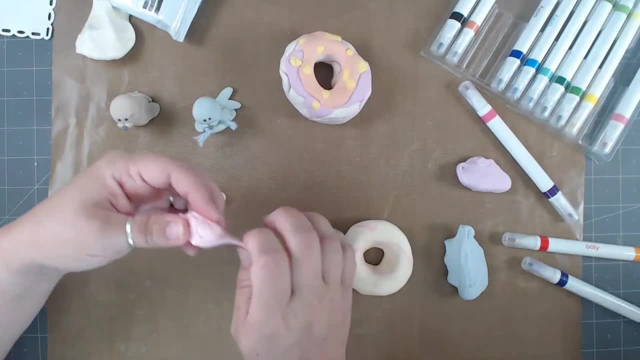 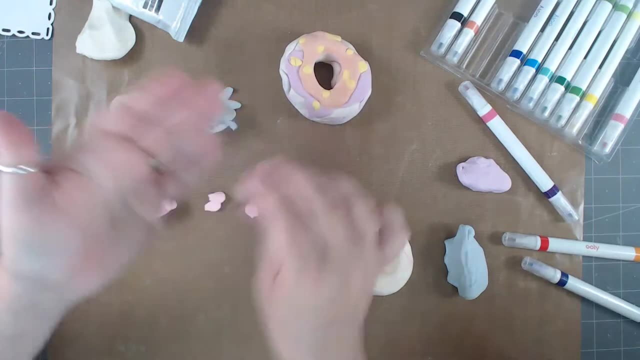 yep, cool ears off. it just did. the arms didn't quite work. I think I made the body too big, so I'm gonna start over. I like the size of the head, though. so, like I said, I've already got all my pieces. I like the sizes that I had. 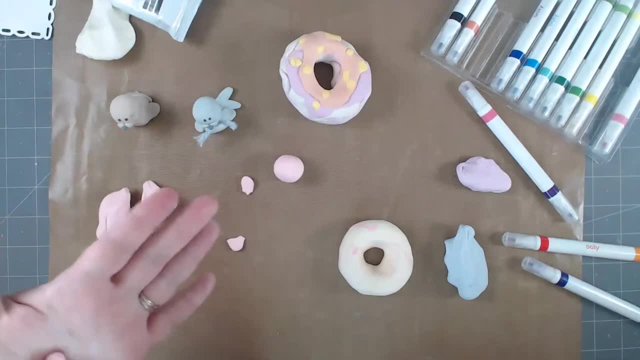 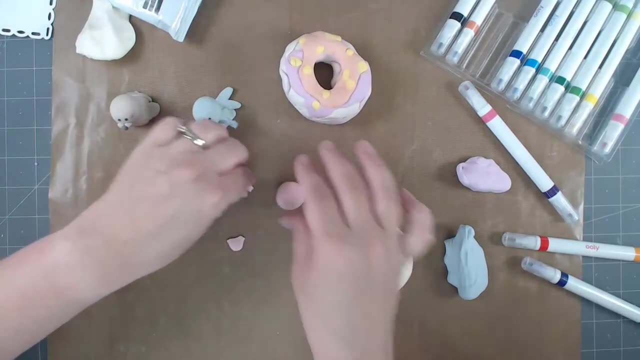 for stuff. whoops. I think I'm pretty sure the bigs the head straight it has to be a little bit bigger than a body, though. I think so I think the head needs to be a little bigger than the body. so I like the size, I like the comparison good. 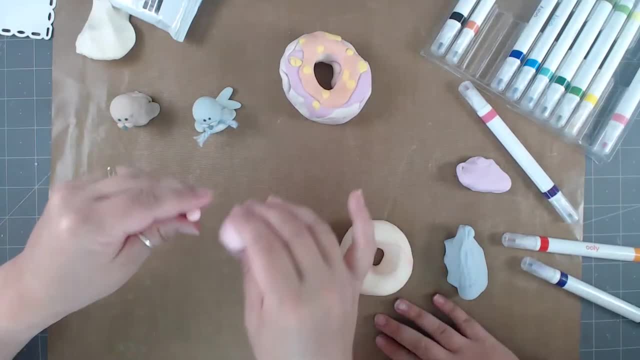 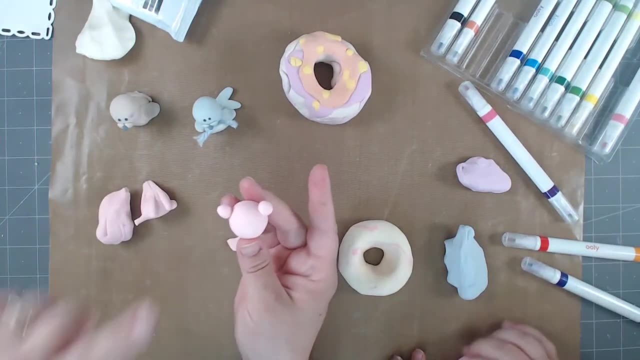 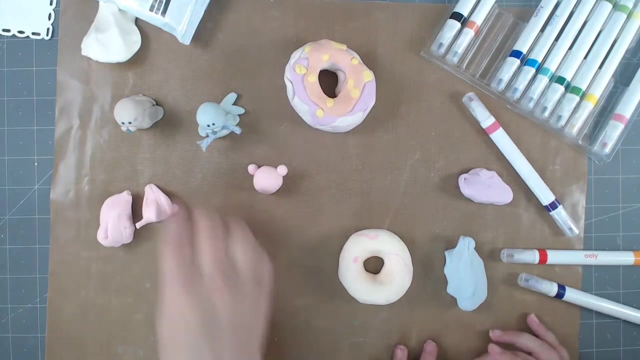 time for to put the frosting on. and for those of you science geeks out there, this is. this is water, h2o- two H's in an oxygen that's you owe. or it could be Mickey Mouse, everyone. look at it okay, and I'm gonna redo my base of. 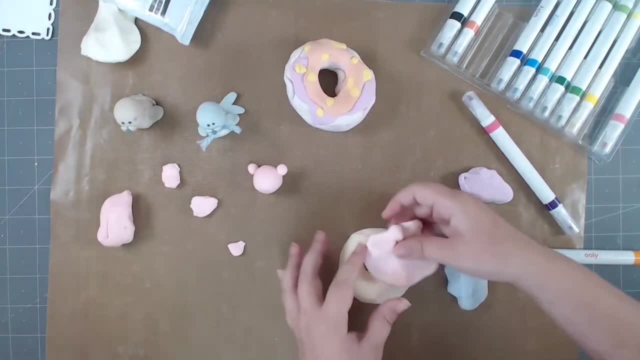 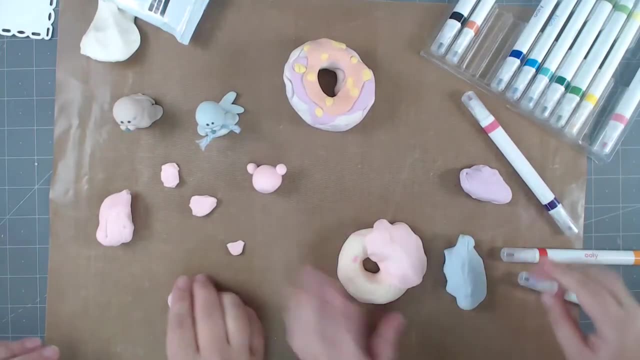 my body. I'm gonna take that back off. I'm gonna make this a little smaller this time. I think I'm gonna build my body before I attach it to the head and I'm gonna do the arms first, cuz that's the part that's the hardest for me. so if you feel like you're like, okay, I'm almost there, but look, 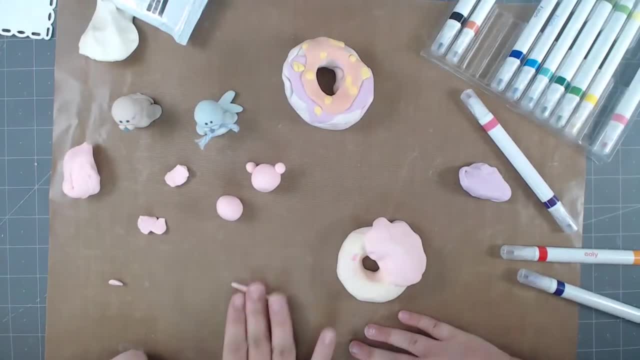 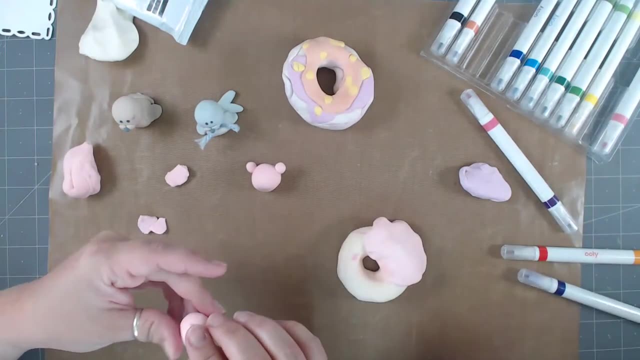 how fast it is to reroll the ball. it's not hard, so I'm gonna reroll this out. I'm going to have a size blue, one half set one blue. one side blue, one side pink. yep, still screw that up. I think the arms are the hardest. yeah, cuz you have to get the perfect. 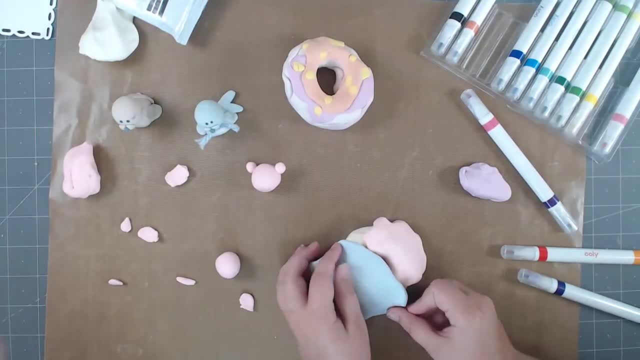 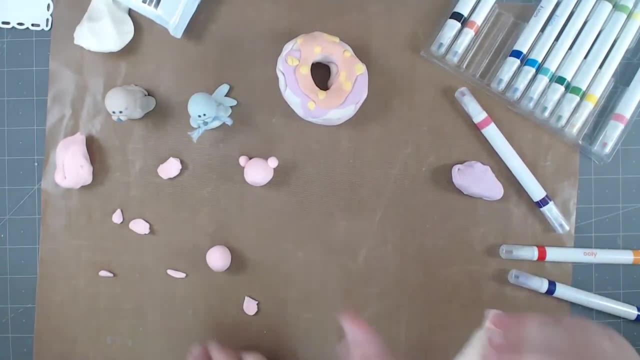 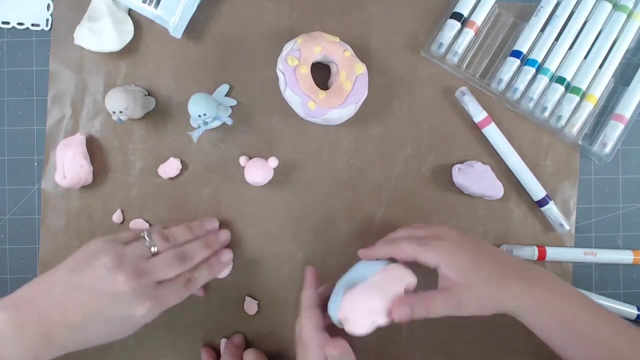 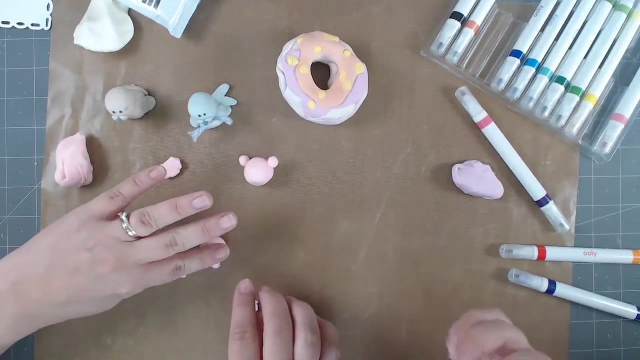 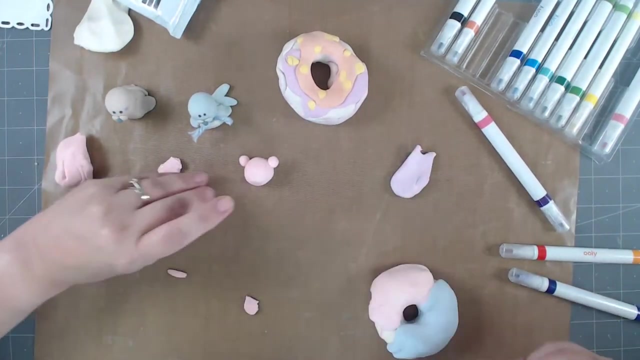 size, right, oh, so it's like frosting going on here. yeah, two different colors, like Harley Quinn- hey, my daughter's seven, she knows who. Harley Quinn is awesome. okay, I'm liking that little arm a little better. what do you think? yeah, it's a good. I have a good. 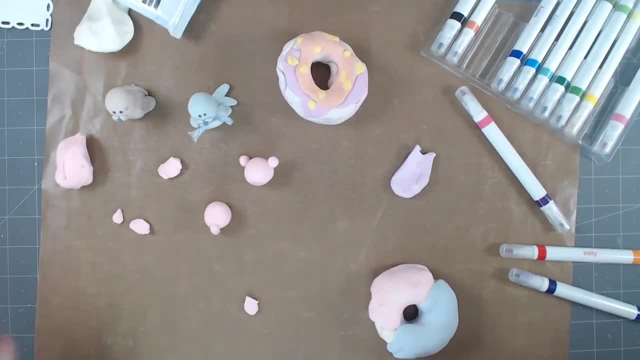 arm. all right, so I just make another one that looks just like that. I don't think that. I think the body's a little too small, though well, I think I want the smaller body, then we'll help it work better. I'm adding purple on the sides. 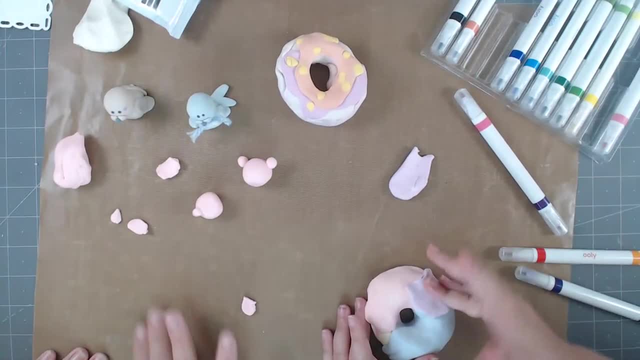 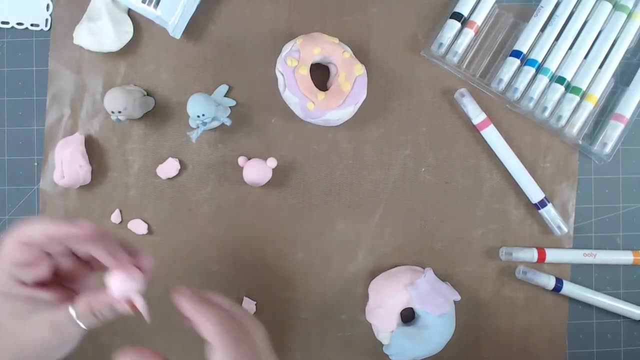 okay, one little arm. arm needs to go all the way to the bottom. I'm not actually making the same donut as that one, but I'm making a donut. oops, when I made these guys, you know how many times I ripped them up so many times cuz I was like, oh, this is not working quite right, this doesn't look. 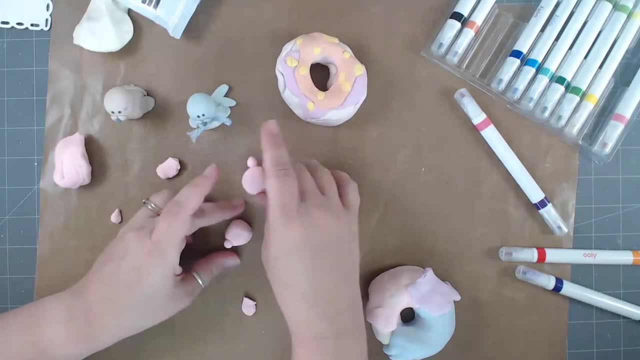 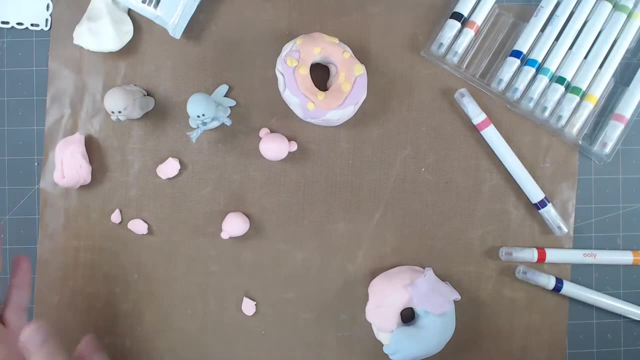 right, right, it's a little too small, well, and now I can kind of I like that. that looks good. okay, let me get this other arm on there and then I'm gonna do the other arm and then I'm gonna do the other arm there. she likes the blue and pink frosting. she thinks it looks good adding purple on the side. 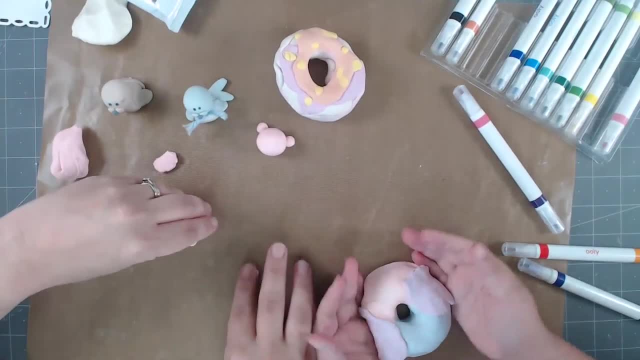 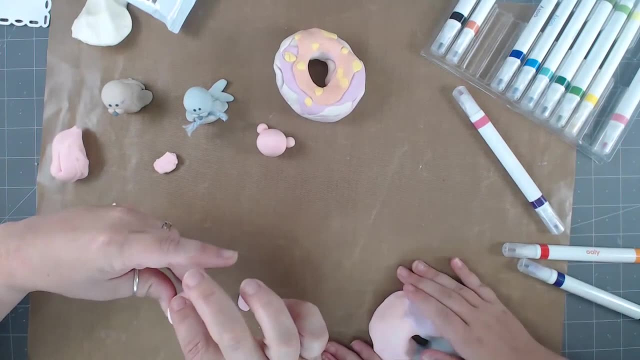 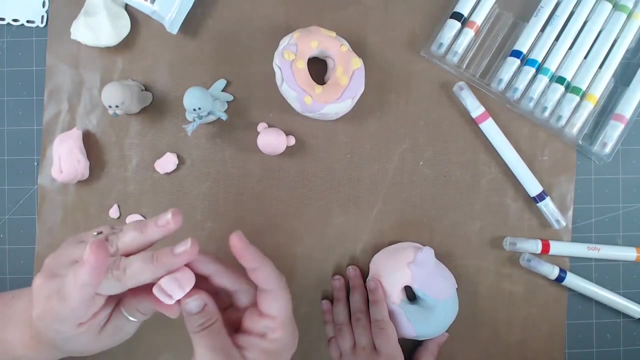 am I doing it? it's done, but not quite done, because I'm gonna go in and draw sprinkles with I don't know what color to use the sprinkles. okay, I'm gonna just draw the sprinkles on, yeah, okay, all right. so there's my little arms. I like those a little bit better, okay. so now we're gonna. 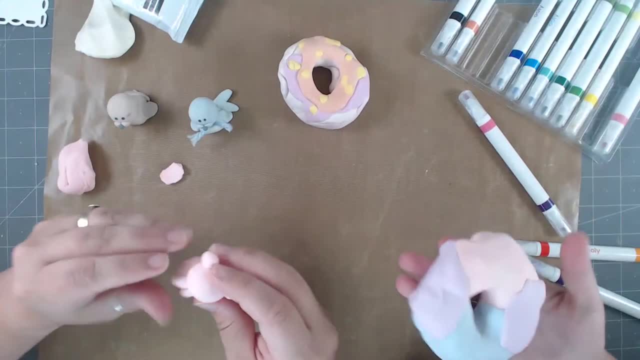 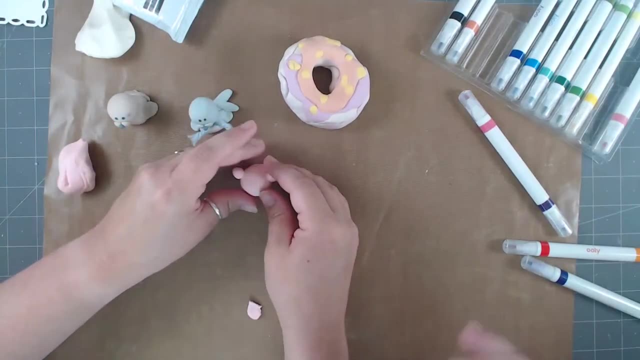 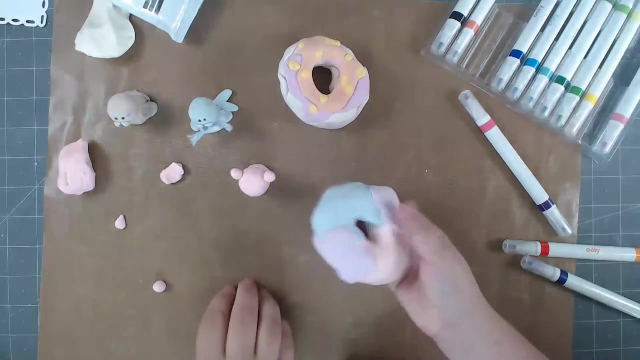 do. that is done, but I have to add those wrinkles look kind of cool, though it looks like real frosting. there we go. it's our legs, that's our front arms. cool, I said the bottom looks like it just has been chiseled. they can't see what you're showing. you gotta show over here. that's a pretty. 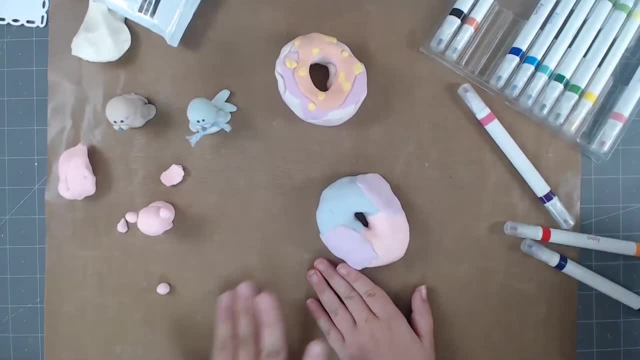 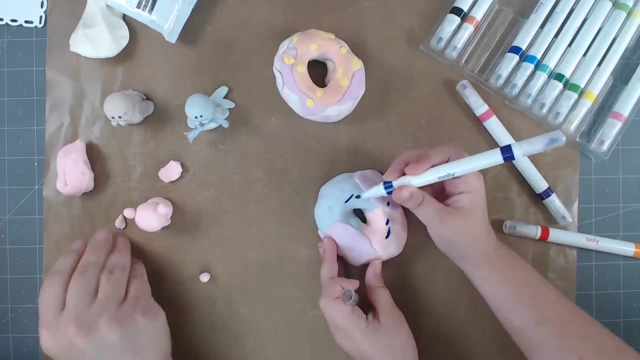 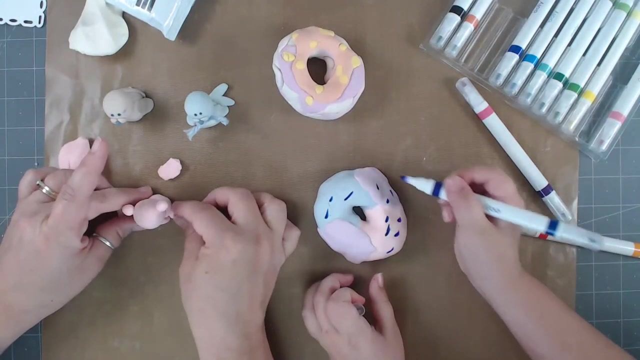 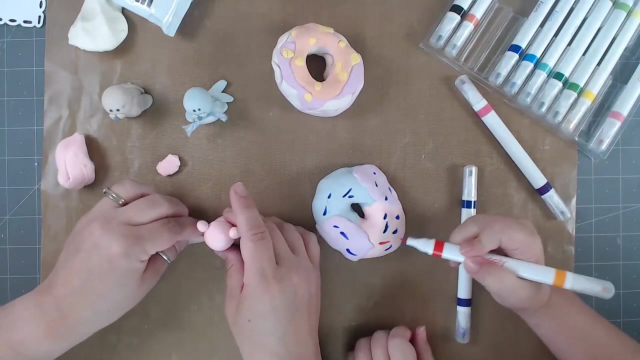 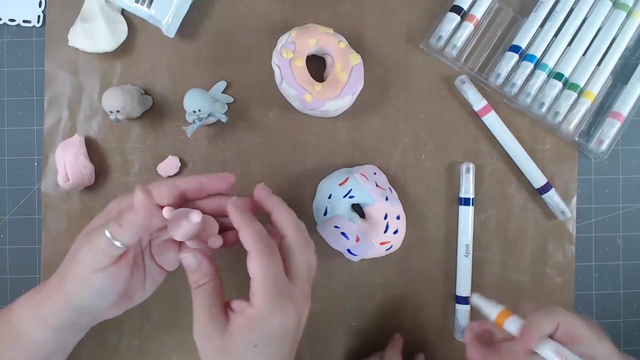 that. oops, that's pretty fun, Catherine. I'm gonna add some different color sprinkles. oh, those are dark. you want that dark? yeah, okay, so she's obviously having some fun here. I'm gonna add my little feet. so here we have little feet, little arms, and then we got our head. that's a little wonky, but it's okay. 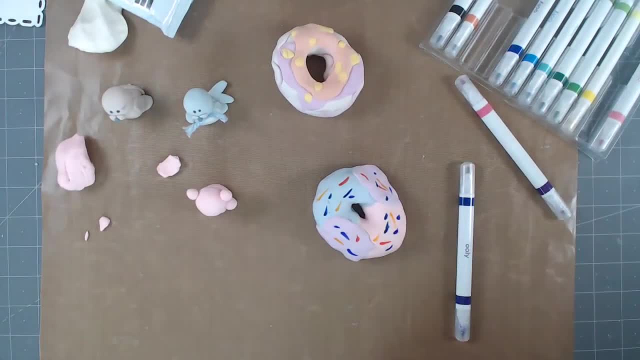 my ears are a little further set back than I'd wanted, but I think I'm good. I don't want to rip it apart at this point, because I like the way that everything's kind of laying out. it's looking very bear-like. now it's just time to add: all right, so now I gotta do the face. so 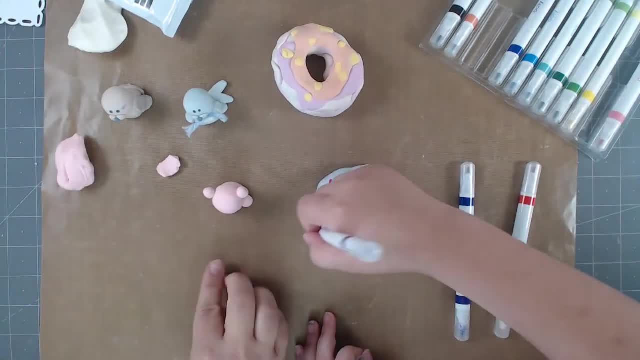 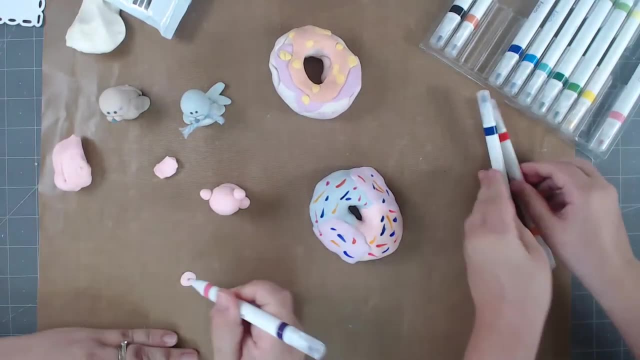 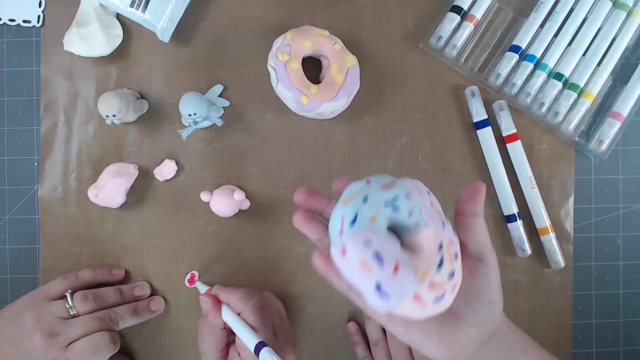 we're, I'm gonna take, and I'm gonna take this little piece right here. so I'm gonna take this little piece right here and where's that pink one? here it is, and I'm gonna add a lot more pink to this and, look, I have enough that I can make a whole nother bear. yeah, oh, you're all done, man. 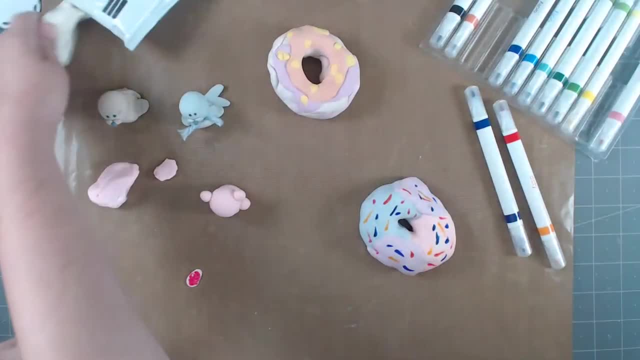 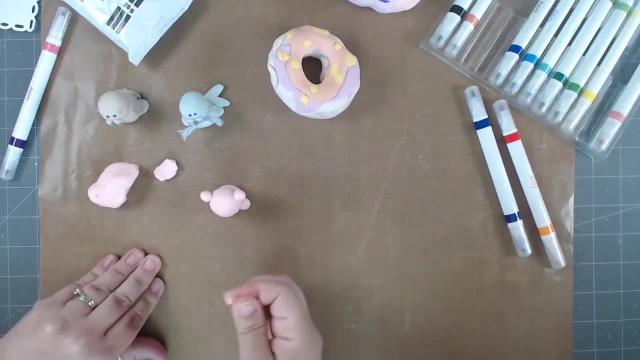 that was fast. you are, yes, one clean over here. so I know, and I didn't use up it, yeah, go for it, what do you think? so I'm just trying to make an even darker pink shade, if you know that you're not going to be using that much. so you could kind of like kind of get all your pieces set out and then 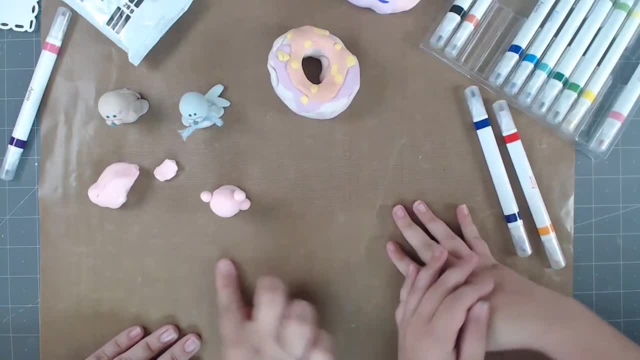 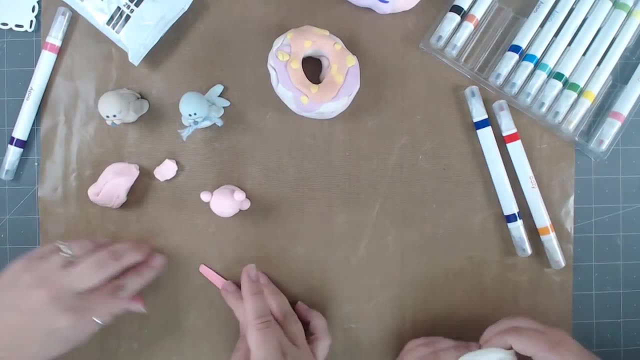 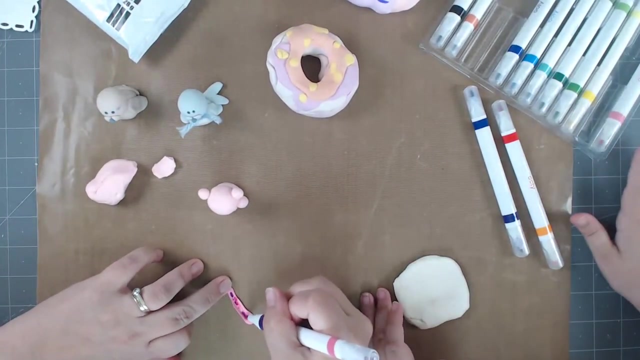 add your color and then you're not coloring. that's like molds and wait for. like you put it in a mold and then you wait for it to dry and then you take it out of the mold. yeah, so, or you could use cookie cutters. that's kind of fun too. cookie cutters are cool. all right purple to this. I think it's kind of. 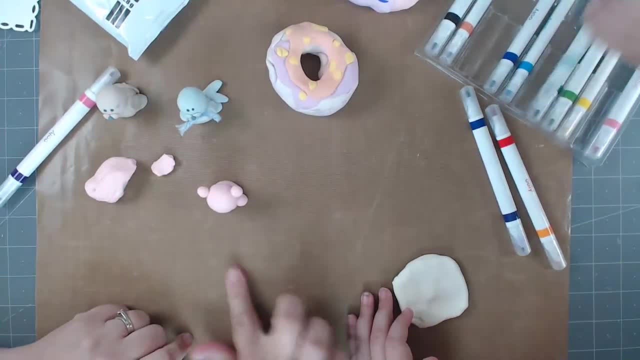 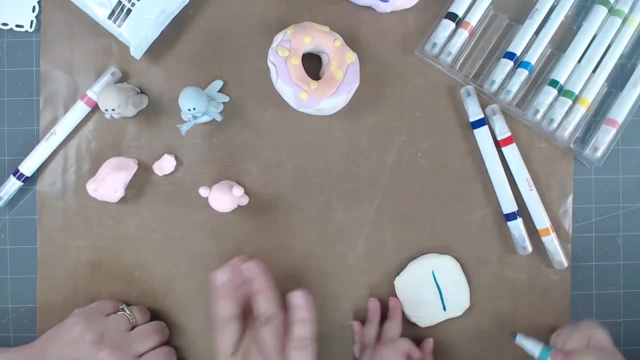 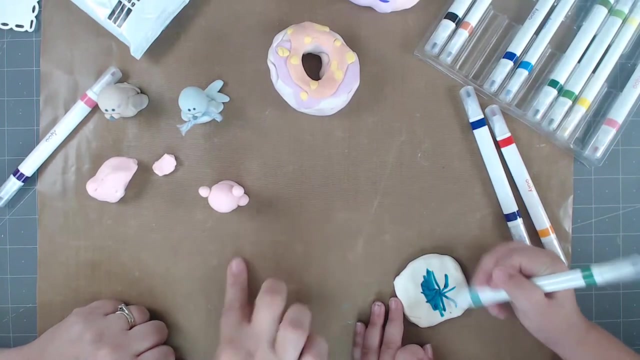 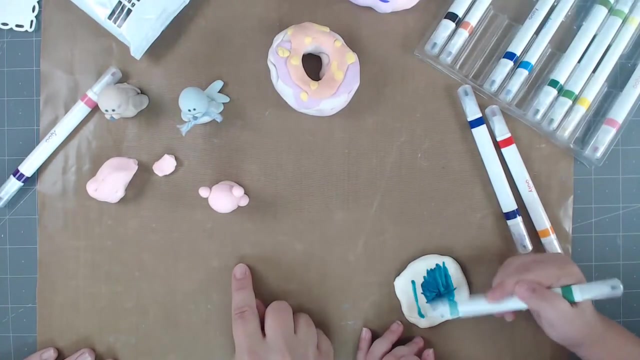 cool when you add a different colors to different types of things, like I'm gonna add, like, like, like green color. that's teal, that's pretty, I like that color. so what are you gonna make of that? you make a fish. yeah, I might make it like a mini soap sheriff dinosaur. sure, all right. so I'm making. 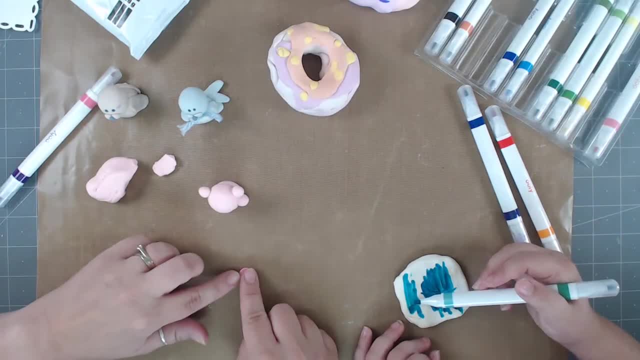 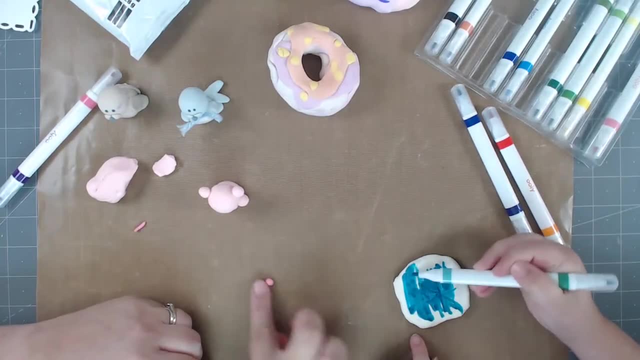 a little muzzle, I can make a turtle. I can make a turtle because I can use the pink. I can use this for my shelf, sure, yeah, I can use a pink for, like, the head. so many options, all right. so what I'm doing right now is I'm making a little muzzle, so I'm just making a little circle and this: 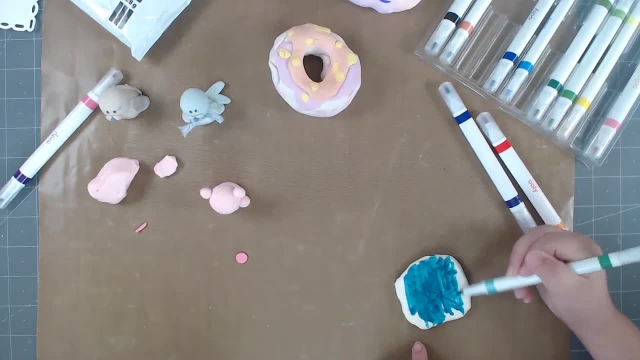 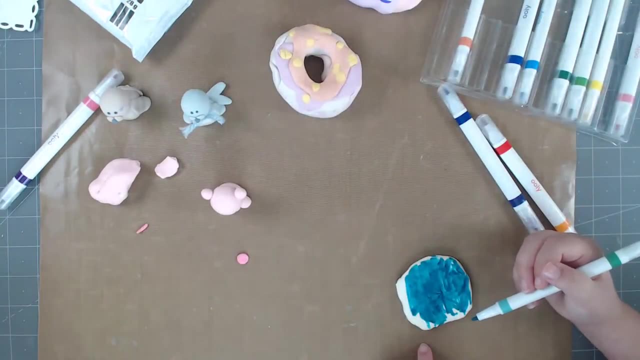 is my hint to you: if you're gonna make little animals, don't try and turn anything black. it's just not gonna happen. so we're going to take the black marker here- actually clay black, you could, because if you put black on there it's just gonna make it gray. so I'm gonna do is I'm gonna draw a. 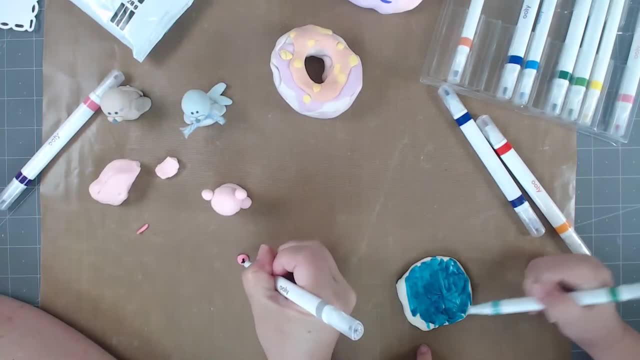 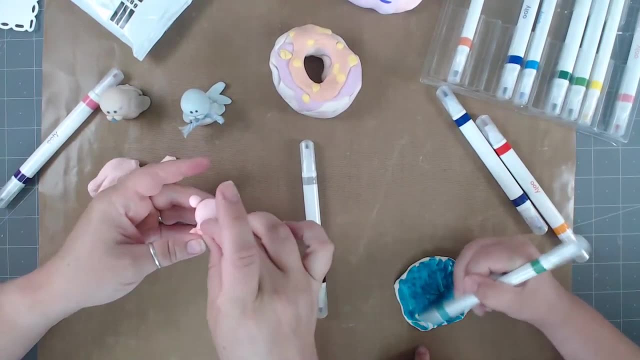 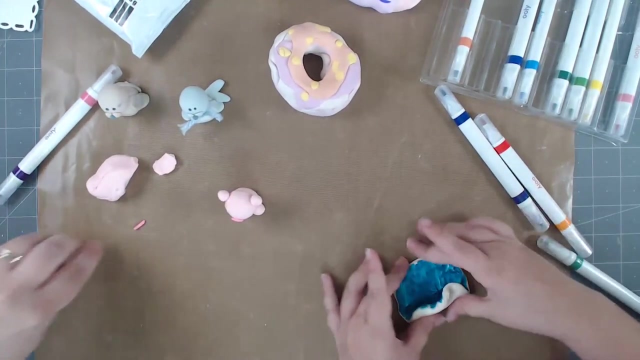 little nose and a little mouth. so that's a little nose, little mouth. now, very carefully, come in and place, because the clay is gonna want to stick. that should be enough. that's his little mouth, and then I'm gonna come in and draw the eyes on there. so, and I'm just gonna kind of so just to show you this is how I do. 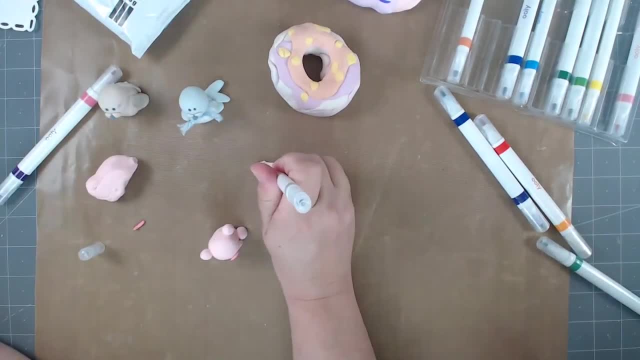 the eyes. I just come in because I don't want to mess this up. I just come in and I push, and then I push. you don't actually try and color it, you just push it in, and if you do that it has a really good look. so where's the eyeball gonna go? 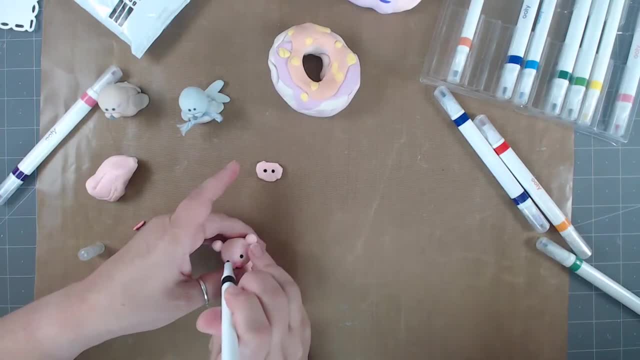 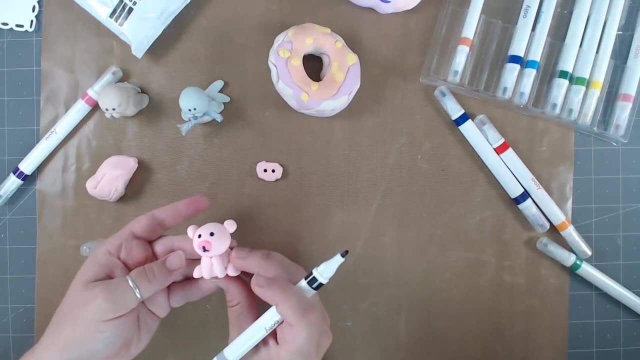 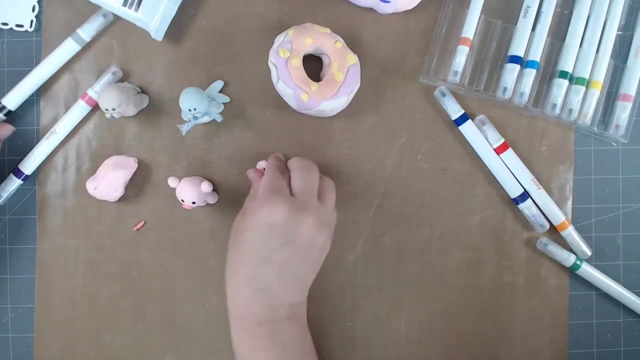 why are you doing two pushes? oh, because that you're just showing them how to do that right there. yeah, and there is our little pink bear. adorable pink bear. it could be a white bear, though you can make it any color you want. yeah, I mean, you could make this a polar bear that kind of looks like a pig, a. 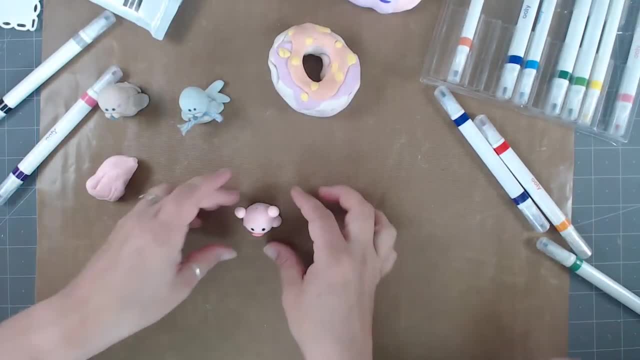 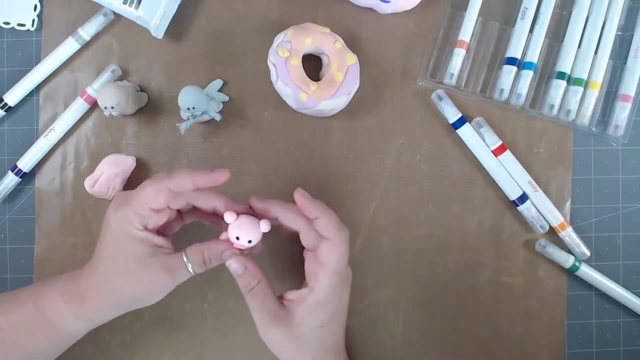 little brown. sure, we could go with because it's pink. it makes you think, yeah, you know, whatever it looks like a little bit of pig. if you put brown spots on it, it looks like a real pig. so you could definitely do a pig. I could change the ears. well, should we do that? should I change the ears to make? 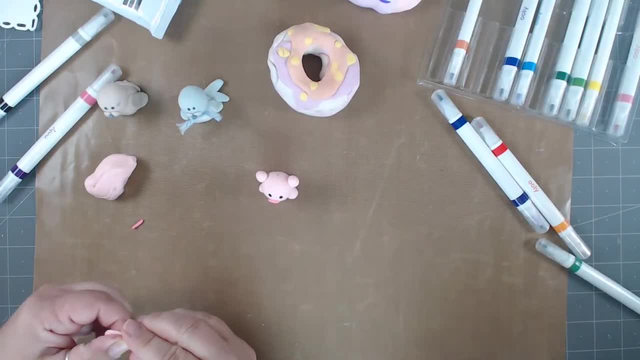 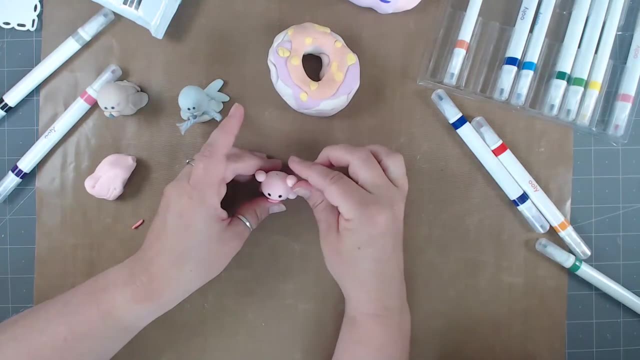 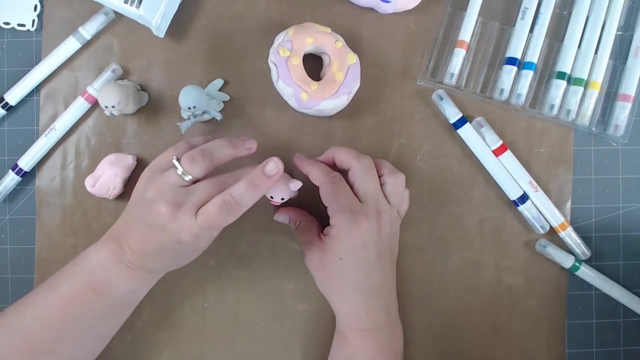 it look more pig, like: so what would a pig ears look like? uh, pig ears have like: well, they're kind of pointy like that, right, yeah, yeah, okay, so let's change. and I think you should want to add: like a black spot so it can bend in the dirt. make it bend in the dirt like I'm leaving my pink. it's my pig. 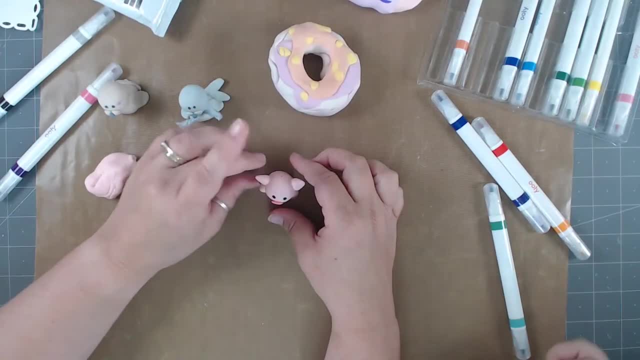 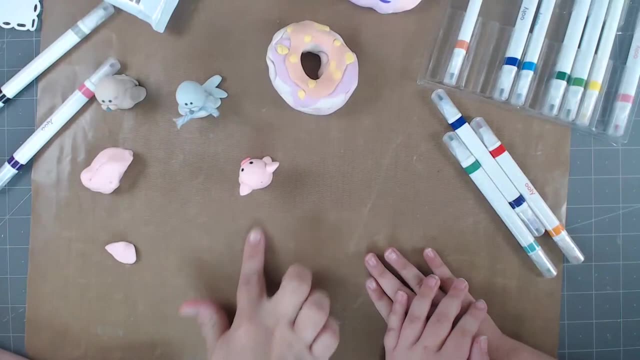 so look, we just went from bear to pig in two seconds. yeah, there, does that look like a pig now? yeah, so now you can add a little curly tail. oh, I got this little guy right here. we're gonna add a little curly, cute tail. I told you you can make different, like sculptures out of. 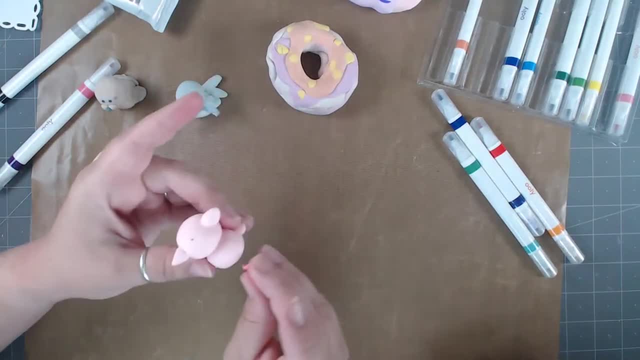 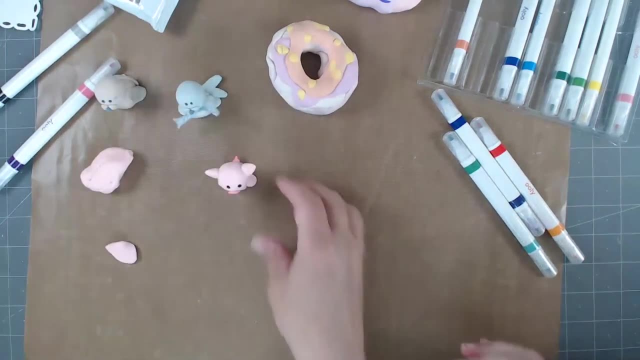 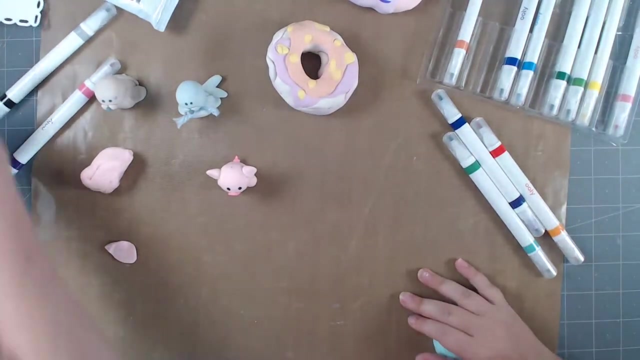 like you made something and then you could turn into something else. yep, there, that looks like a little piggy tail. yeah, awesome. and there it is. we got our little piggy. I'm still making my turtle, so what are some other animals you could make? I like my little pig. I think that's kind of cute. 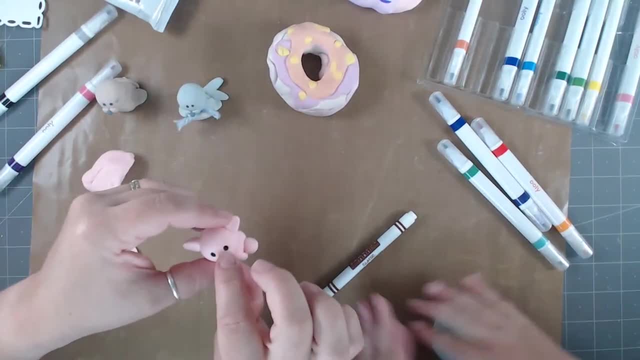 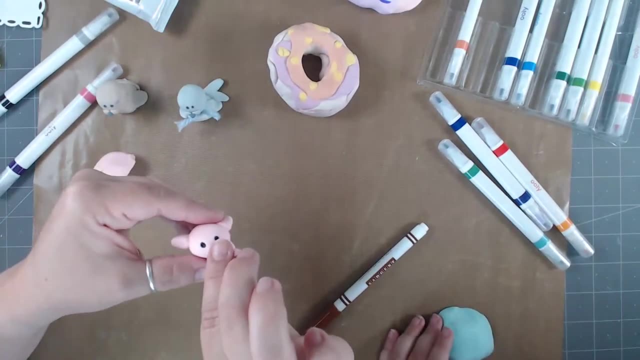 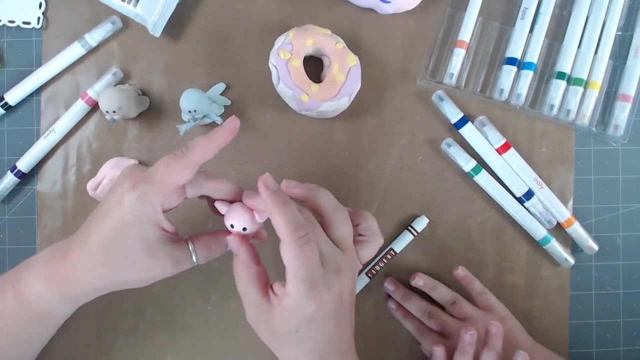 that it turned into a little piggy. of course, the nose should look a little different. if we're gonna do a pig, yeah, it needs to be more like roundish. yeah, see if I can tear this off, okay. well, a piggy snout looks a little bit different, yeah, but that looks okay, okay. well, I'm gonna fix it, I'm gonna. 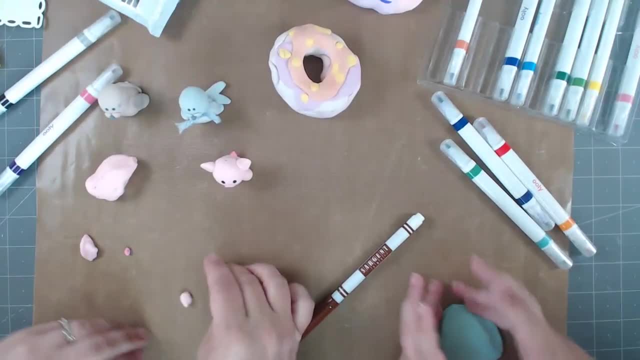 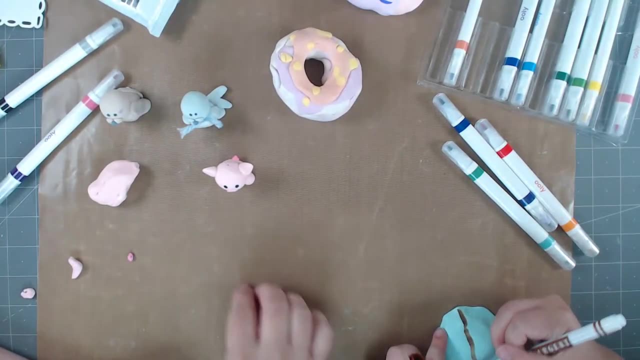 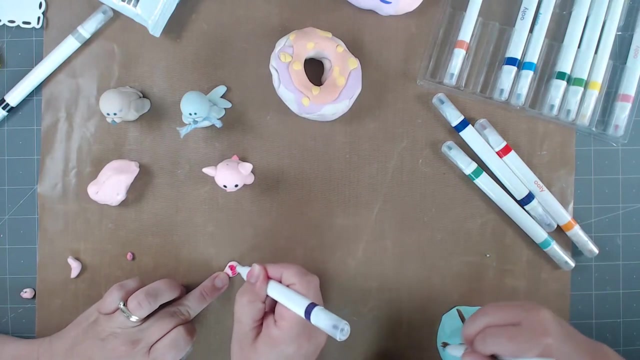 take another piece of this and make it hot pink. all right. so remember a piggy snout. I'm just gonna make this more hot pig, so we're gonna fix our pig real fast, because a piggy snout is got two dots in it, right, yeah, all right, so it's just two dots. 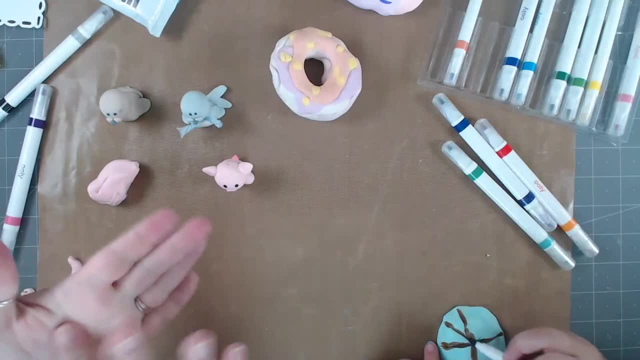 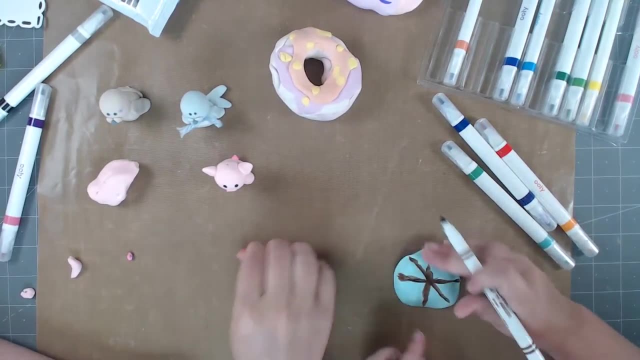 you know turtles back and out and design on it. yeah, it's true. so we're amending our little piggy here. yeah, man, so that's. the cool thing about clay is that you can always rip it off and kind of start over, and then nothing is set in stone. 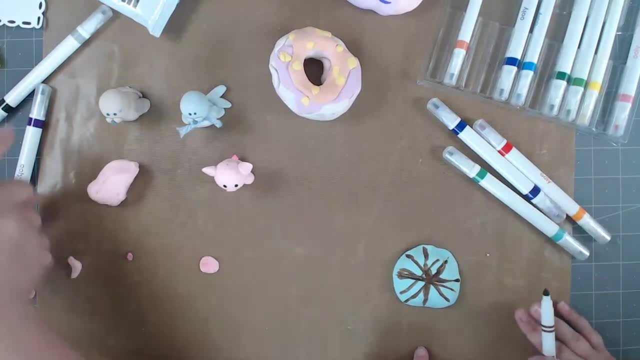 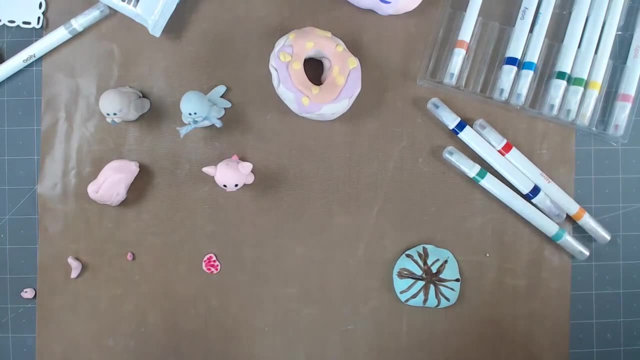 that is the awesome part of it. unless you put it in the oven, it will make it dry off. this is not oven clay. it's a good point. there's different types of clays out there, and this is an air dry clay, so this is not the kind that's meant to go in the oven. all you have to do is make it warm. 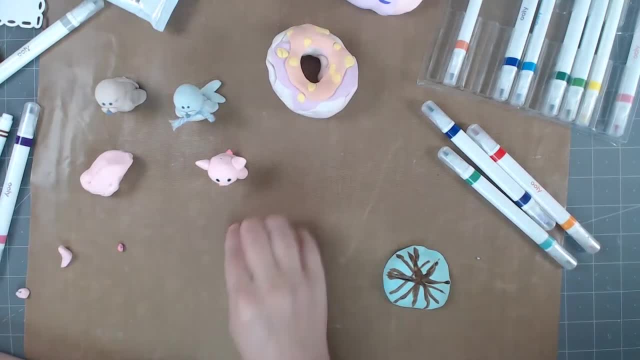 and it'll start like you can play with it forever and it won't dry out unless you put it in the oven, right? so you're. there's some clays out there- sculpey is one of them- where they cure in the oven, and that's not the kind of clay this is. this is a truly an air dry clay and you can get. 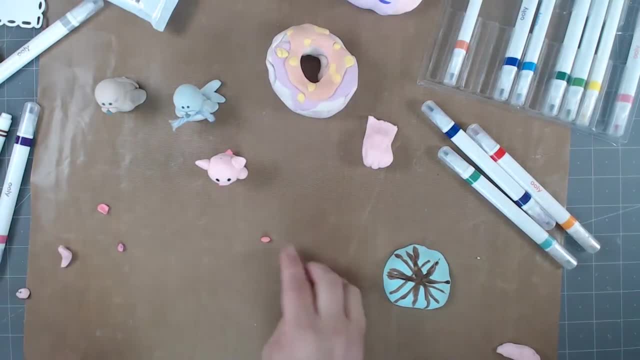 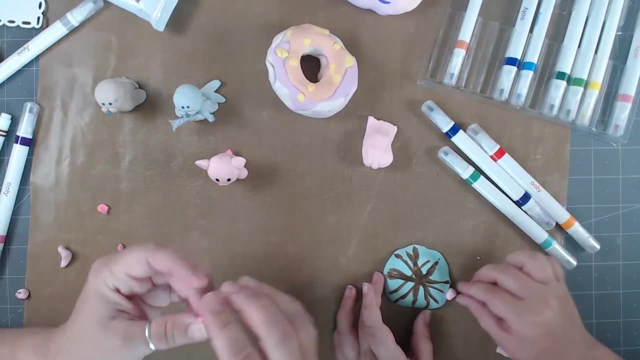 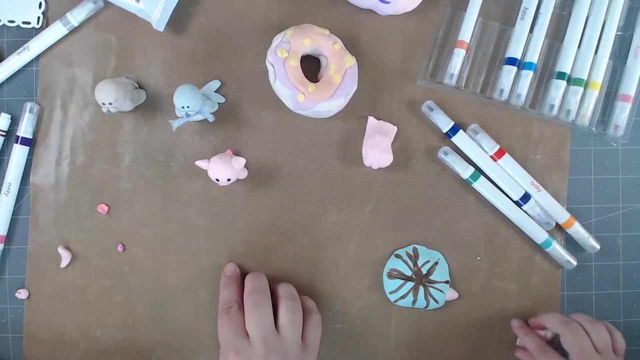 these packages at a much bigger. they're like really giant, and so these little little guys right here and there are colors already, so you can find this stuff lots different places. I'm just using you called already have to make them. yeah, sure I like it. make sure you don't. 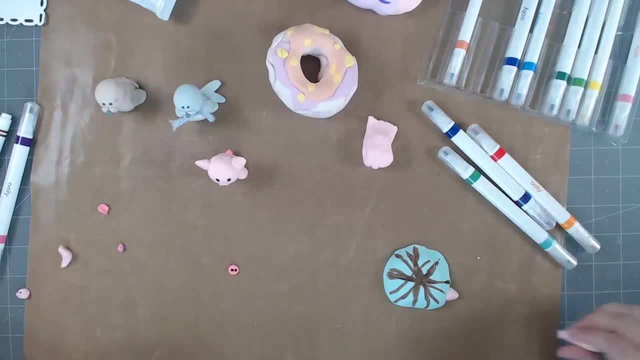 make the legs too small or too small. if you don't want to make the legs too small or too small, make sure you don't make the legs too small or too small. if you don't want to make the legs too small or too small, big because you have to have that. look like a piggy nose now. yeah, all right, there's our. 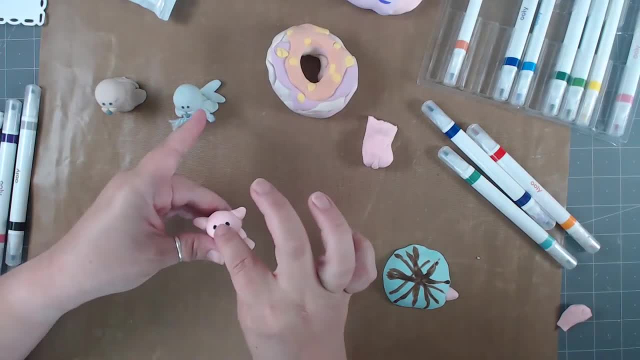 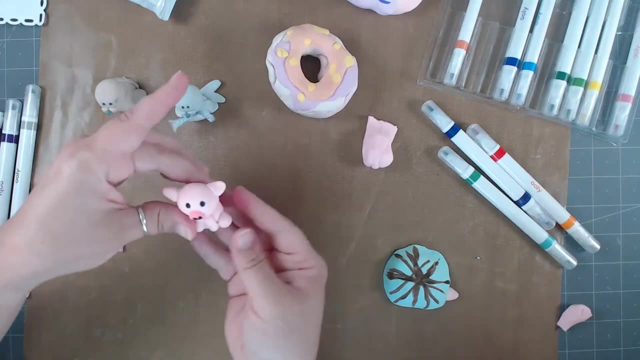 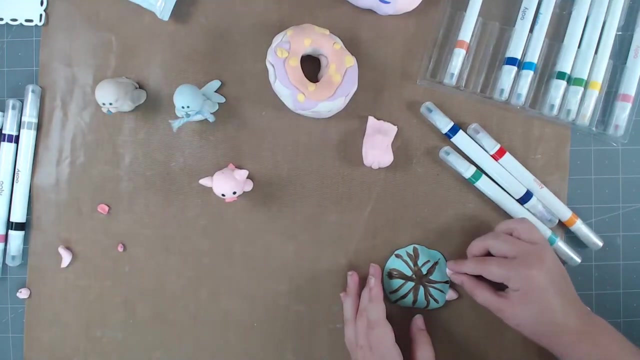 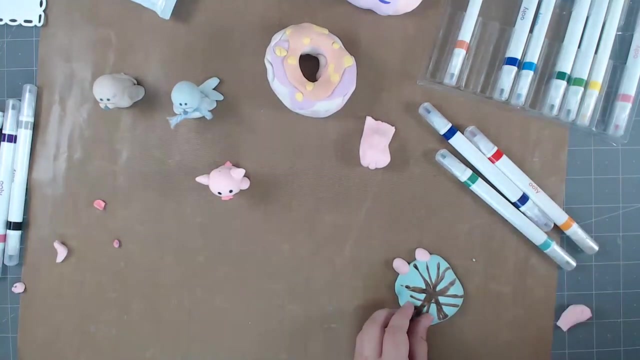 feet. you know this and I'm gonna cover up. yeah, so now we have a piggy that look like a pig. now, yeah, you got a little smushed. the more you mess with it, the more that I get smushed. now we have a piggy, but I usually bear and go pig yep. well, you can turn the pig into a bear, I can. 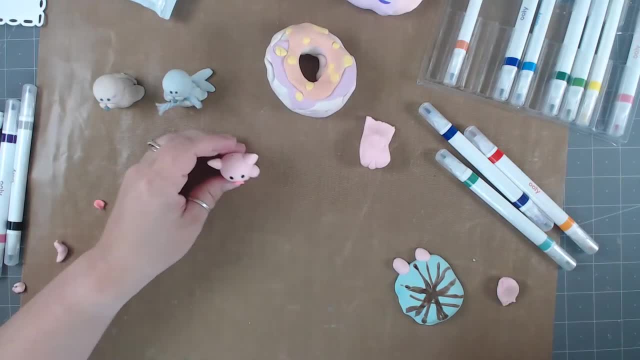 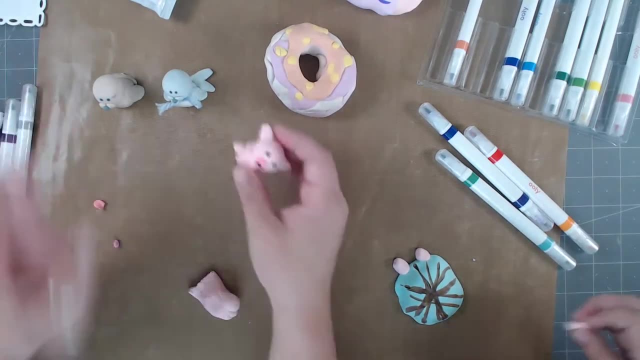 have gone. yeah, so we just, we just amended, and that's the fun thing about clay. she said pig, so we went with pig. but yeah, I could totally make something else and you could do it. I'd like, for some reason, I kind of gravitate obviously to this size because it's they're quick, they're easy, this. 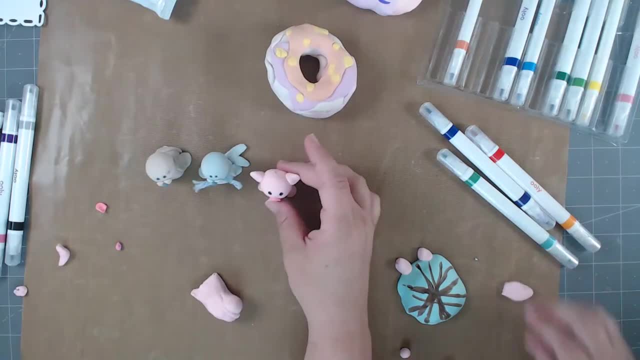 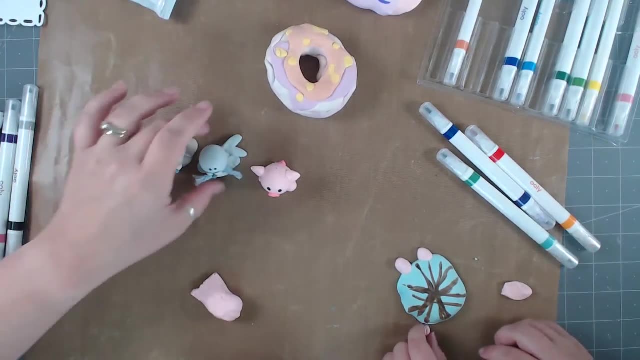 little guy is going to dry. I think they're super adorable. I mean, who doesn't love a cutie little animal? and all of those little squishies are out there right now. so this is like you're making your own little squishy and own little creature. you can obviously add stuff to it, like I add a little. 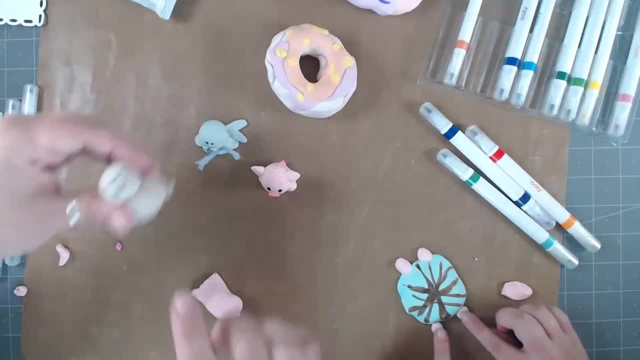 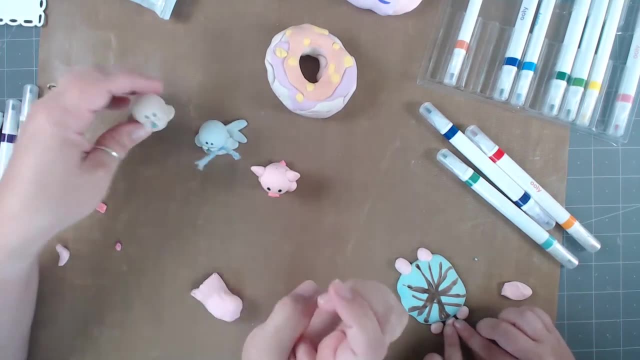 yarn necklace on this guy. um and for, like the walrus here, it's like three different little colored balls, two little sticks right there, and then I did the same trick with the eyes, where I just poked in, where that is, obviously you can add ears. I think I made a polar bear as well. that one was. 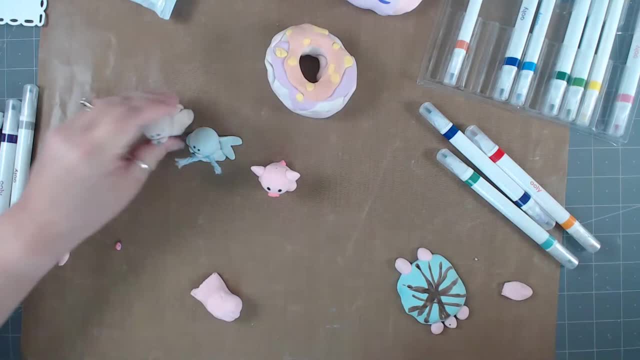 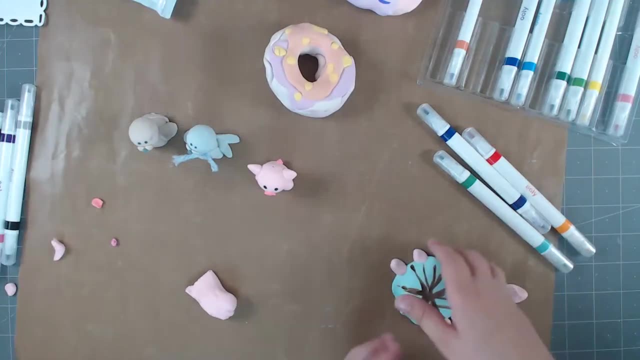 kind of cute, but you guys destroyed my bear, my animals- these are the only two, and this one had a little bit of a- it lost its tail- and a little turtle- that's a cutie turtle, Catherine. I love it. I could sit here and make little creatures all day. 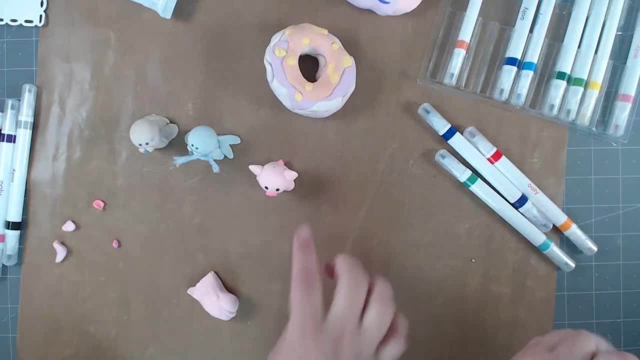 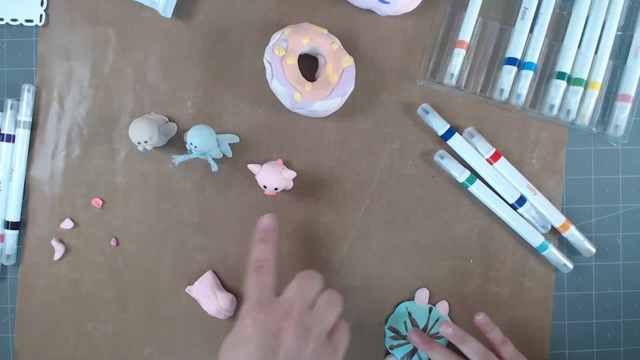 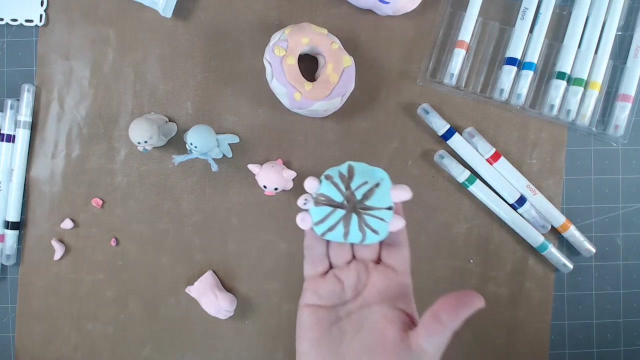 I could have so much fun with this because it's seriously. it's a head and it's a body, it's legs, and then how you treat the color of the animal and also, um, like what shape of ears and stuff, and how you do the mouth. when you put the eyes on, don't make sure they don't mix in, right? oh, look at her. 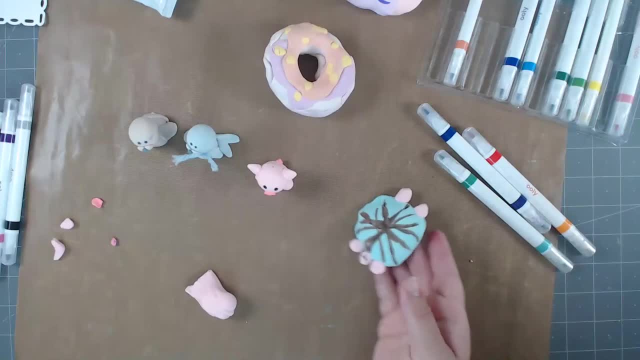 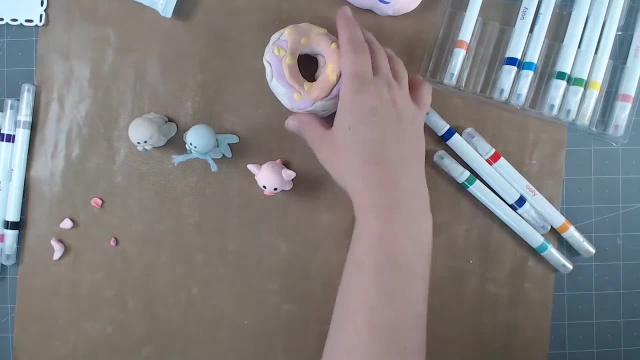 cute little turtle. see, look, she had so much fun. no, the markers. as long as you go, like I can wipe on this and it won't smear. and the other thing is is that you could wait for this to 100 so she could go in now and if she didn't, she could go in, and she could go in, and she could go in and she. 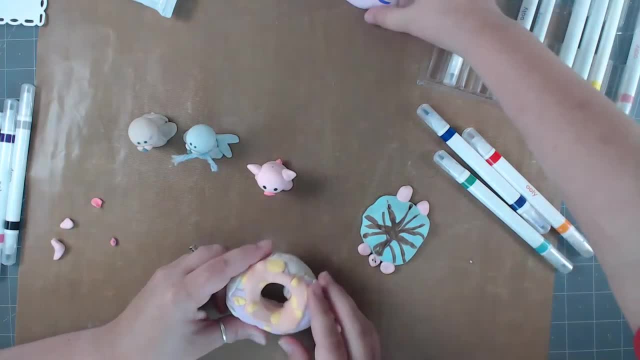 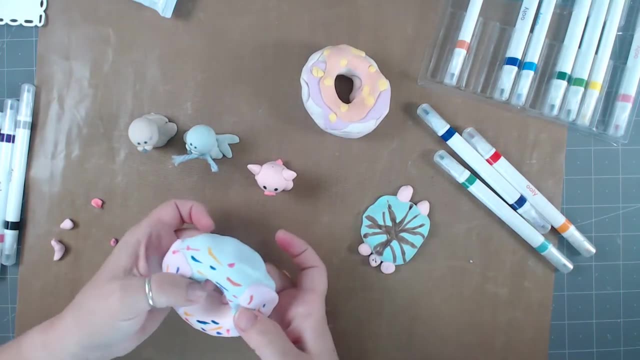 wanted to add, like some other, sprinkles on this. when this is dry, she could do that, so she could color this now, or she can do it when it is trying to drive. oh, careful, careful. so here it is. so here is her giant donut. she's got two giant donuts. it's almost like, almost true that one's bigger. 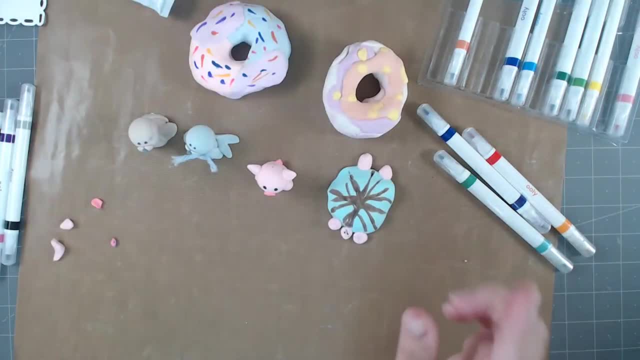 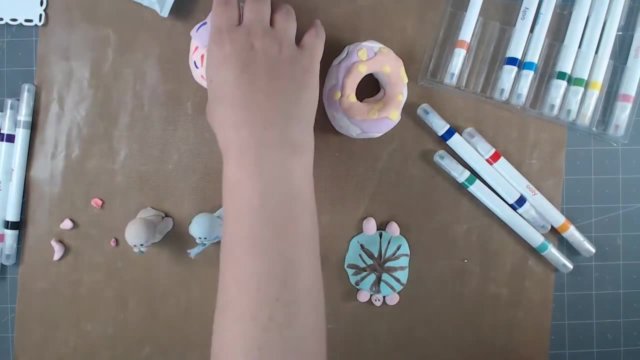 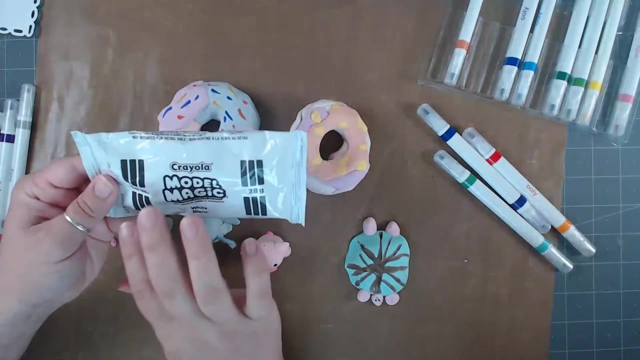 so fun little creatures and things to make. here we've got turtle. usually when you have your donut base, it usually when you put the plastic on it looks a little bit more bigger. yeah, so make sure that you don't say it looks too small. so check these out. these are. this is the mull of magic and this one is not. 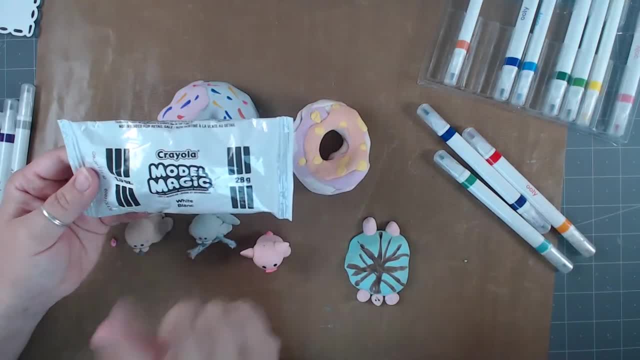 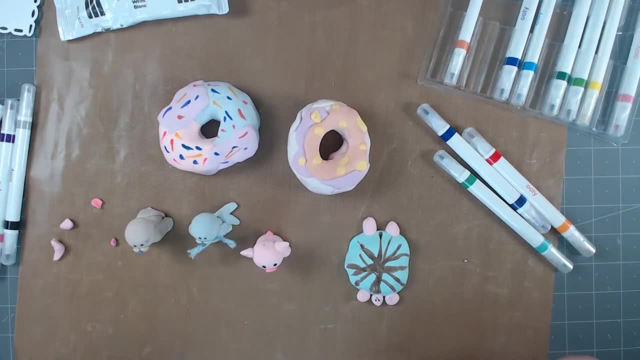 intended for resale. this one only comes when you get packages, um, but this was in the orange art box, which is awesome. you can get bigger packages. I will link to the bigger packages and there's colors you can get. or you can use your markers. I love these ollie ones because for 12 markers you 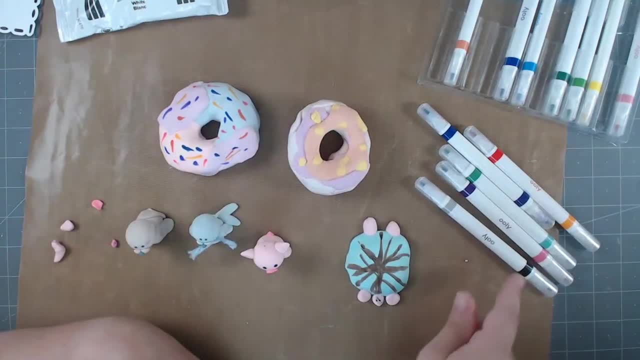 actually get two different, two different colors. you're getting 24 markers in one set and, as you can tell, look how well it colored up this little pig. this little pig is so adorable. I'm going to leave this on my desk. I'm going to leave this on my desk. I'm going to leave this on my desk. I'm going to. 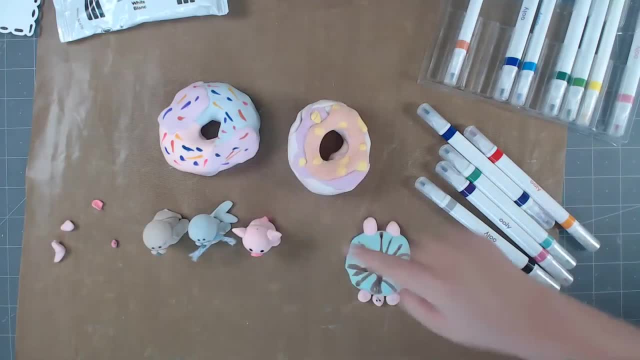 have all my little guys on my desk. now are you going to have my doughnut on your desk and my turtle, sure do you want to put it on your desk in your room? yeah, I don't really have much. you've got a dresser that you can stick. you've got a whole big space with your bookshelf. 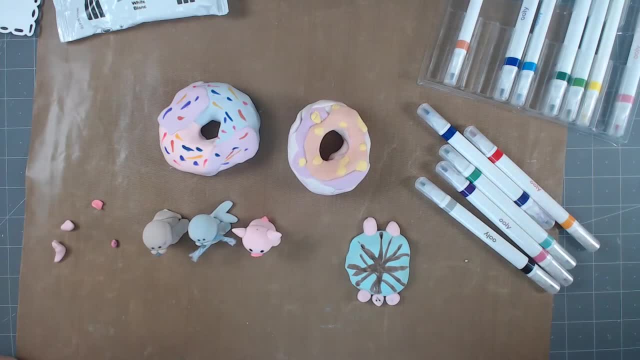 so you can put your little things on I want you to have. yeah, she's giving it to me. okay, that's fine, I'll take your turtle. thank you guys, so much for watching. please give us sometimes up. don't forget to subscribe, and we'll be back next week with some more fun crafts. what are we doing? 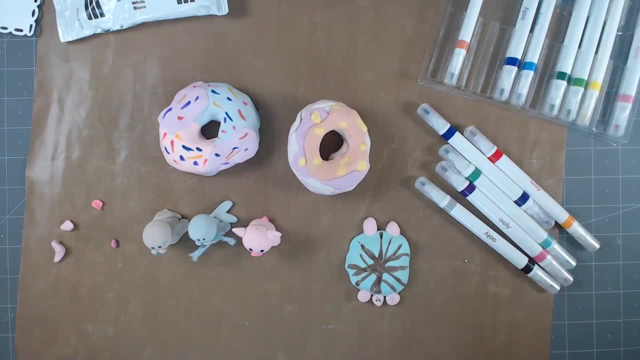 next a week we're going to play it with some wooden slide toys- awesome- and we'll see knives, forks and spoons. so how to take knives, forks and spoons- that could be the plastic ones, but we're going to show you wooden ones and how to do crafts and art with that. right, that's coming.